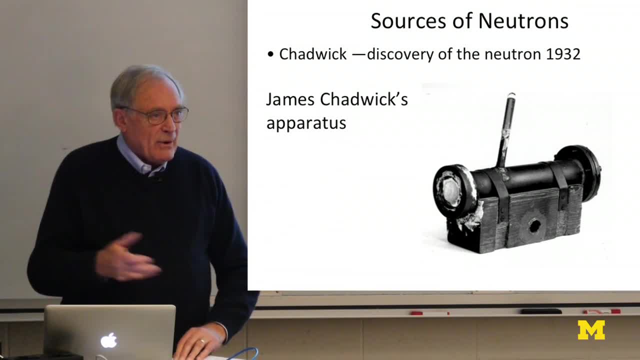 And he could prove that the radiation that came from the alpha particle bombardment of beryllium targets was fast neutrons And they weighed about the same as protons. He came very close to measuring the weight of them And guessed a lot of properties of the neutrons that turned out to be correct guesses. He was a very careful scientist. But his apparatus? what do we have? 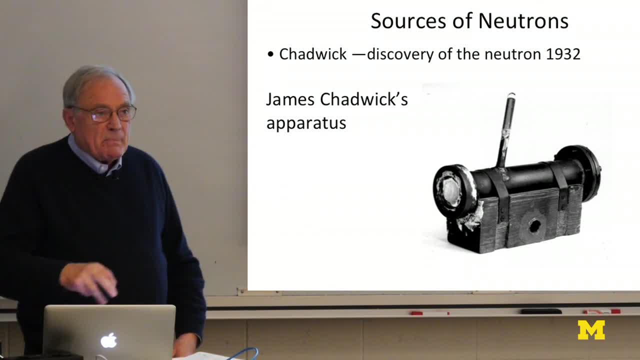 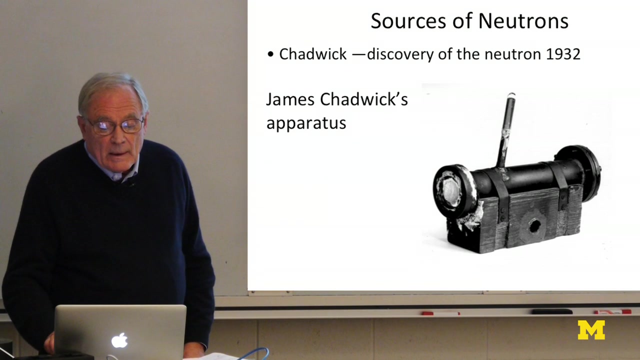 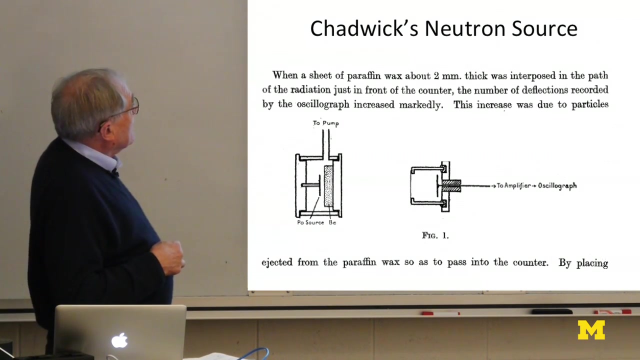 Well, this, This piece of pipe, was his neutron source. Looks like something that I would be pleased to build in my basement. Anyway, this is the way it worked. There was a Okay. yes, He had alpha particles from a polonium. 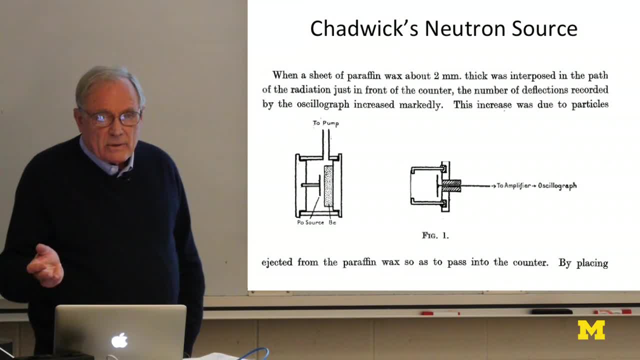 A polonium radiation radioactive source And a beryllium target. You know that alpha particles on beryllium. Now we know that the alpha particles on beryllium give you something like 5 million volt neutrons. So high energy neutrons were emitted from the beryllium target. 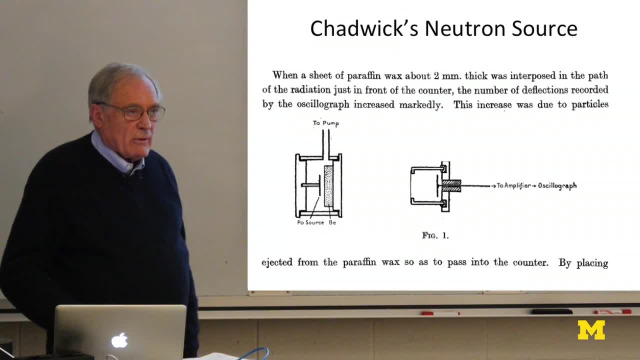 Then he had an ionization chamber, which is just a chamber of air with a Electrodes, So that ionizing particles would cause a current to flow in the ionization chamber, In pulses actually, And he would observe those. He could measure the intensities. 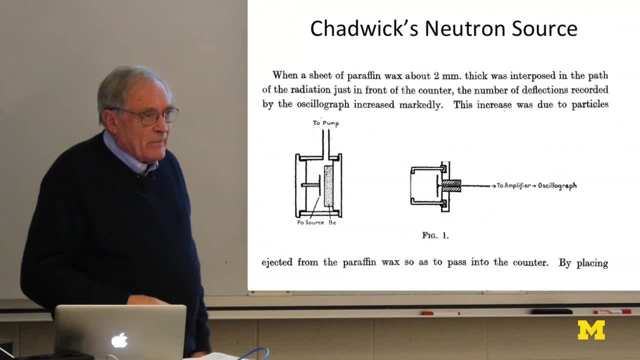 And he made other observations, like: If you put a piece of paraffin in between of here, Instead of neutrons ionizing the air in the ionization chamber There were protons which are charged And they made a lot more charge. 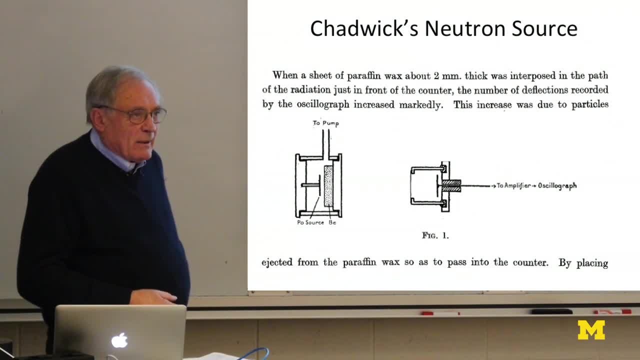 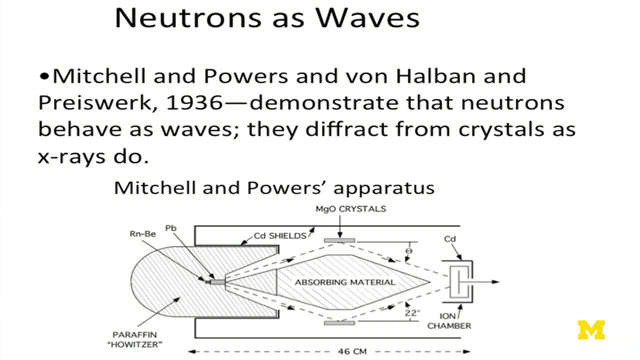 He counted a lot more neutrons just because he converted them by colliding against protons. Clever guys from 1932. That made a big difference in what people understood. So in 1936 people had right to be curious about what are these particles? 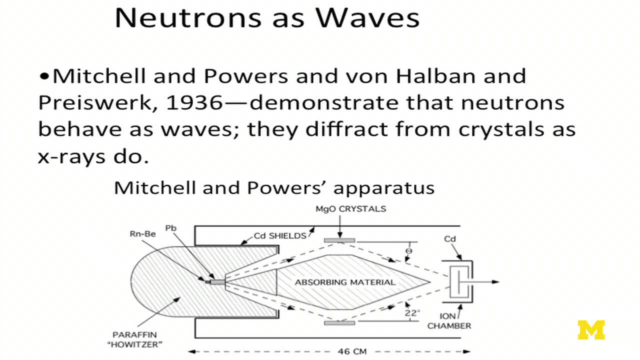 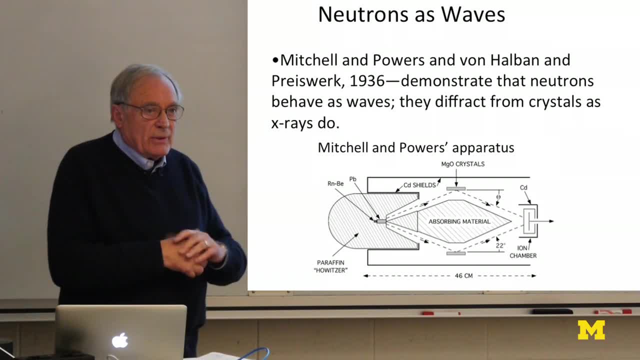 And there were two teams, One, a pair of Mitchells and Powers And another from Halban and Pyserk, Who built apparatus about like this That showed that neutrons diffract like x-rays. X-ray diffraction had been known and understood since 1913. 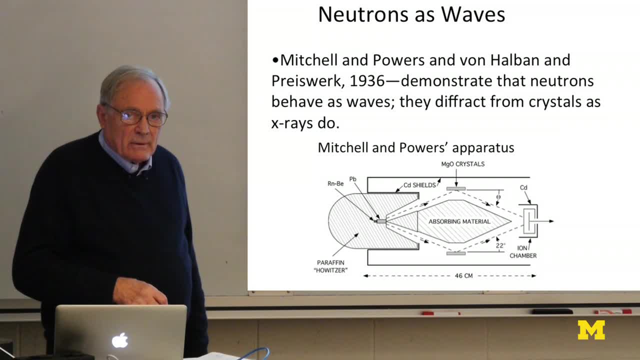 This is the year. I think this is the 100th year of diffraction. Next year, The American Crystallographic Society will celebrate The 100th year of diffraction. next year. Anyway, x-ray diffraction was known And they proved with this apparatus, by changing this angle. 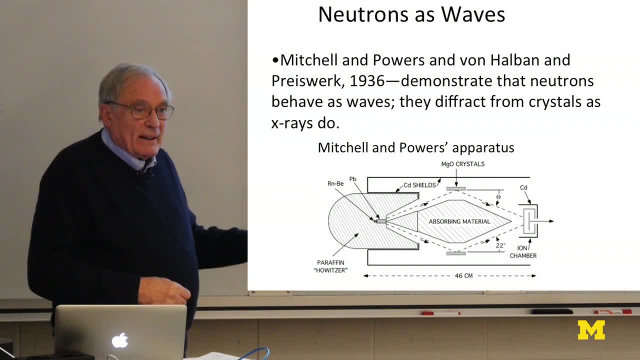 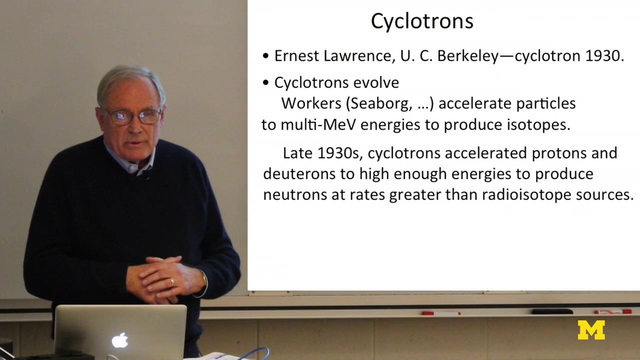 That the neutrons either reflected or did not reflect, According to the new reflection angle from magnesium oxide crystals. So now it was known that neutrons have wave properties as well as particle properties. All of this stuff was done With radioactive ion sources. 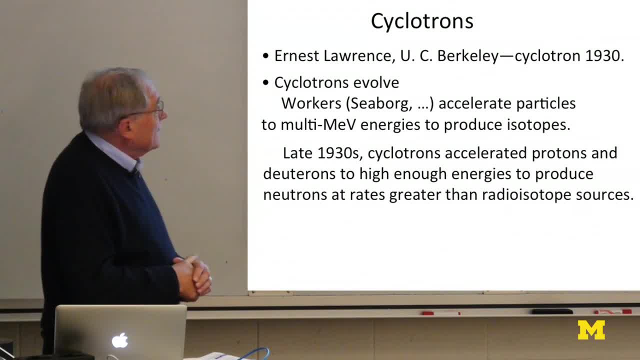 Alpha particle sources And not too long after Ernest Lawrence developed the first cyclotron, Which is about this big. In 1930 people began to accelerate particles, But you needed a pretty big cyclotron To get energies high enough so that particles that you could accelerate. 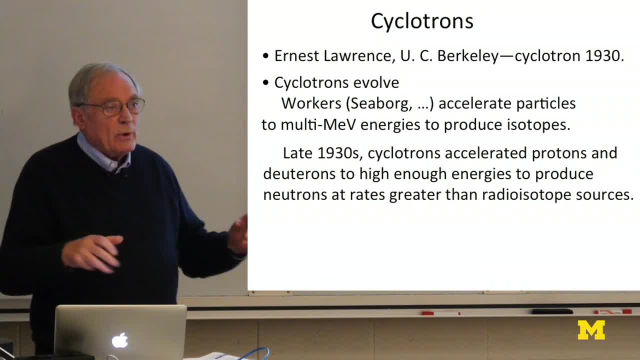 Like protons or deuterons, Would actually penetrate Some nucleus. So it took a few years Until people began to produce isotopes By these interactions And began to produce enough protons So that you had a fairly sizable neutron source. 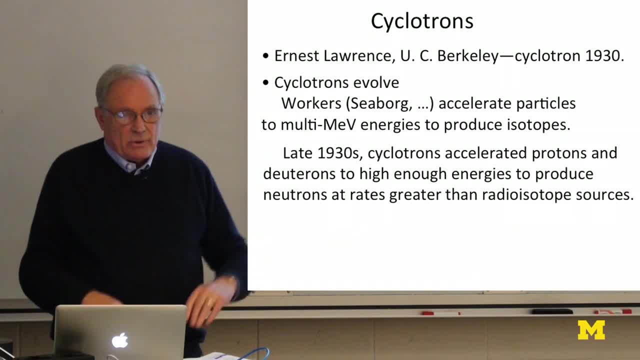 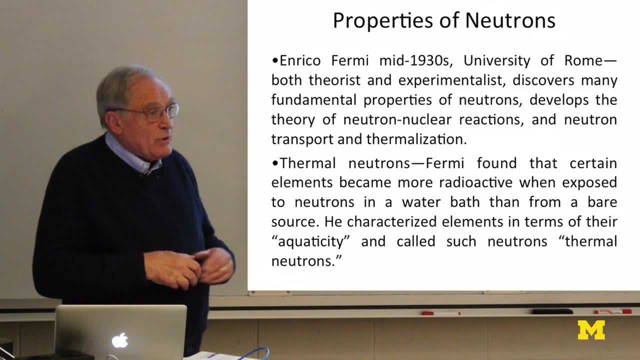 The cyclotrons, in other words, beat the isotope sources Fairly soon. Now, While all of that was going on, People were delighted to be fooling around with these new particles That had been discovered, And Enrico Fermi was one of those, working at the University of Rome. 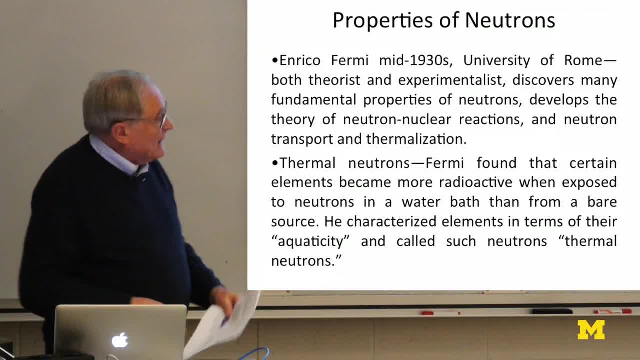 And he discovered a lot of stuff. How much? What did I mention here? Fundamental properties of a neutron, That is to say Their transport properties, That they slow down By colliding With, Say, Room temperature materials And when you? 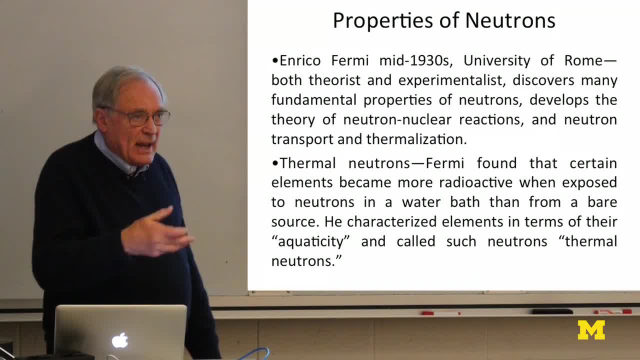 And they activate Neutrons, activate Otherwise substances And make them radioactive And he measured the rates of radioactivity That he could produce And one of the things that Was interesting to me. I think you find this out If you. 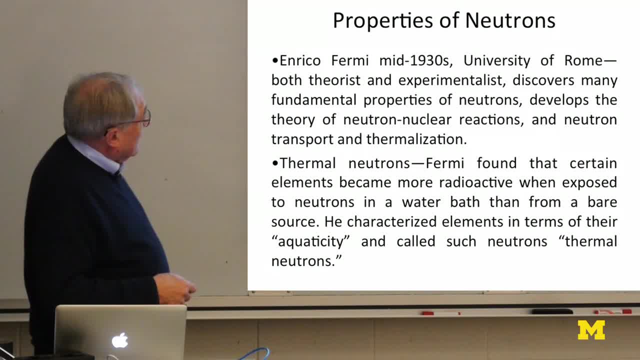 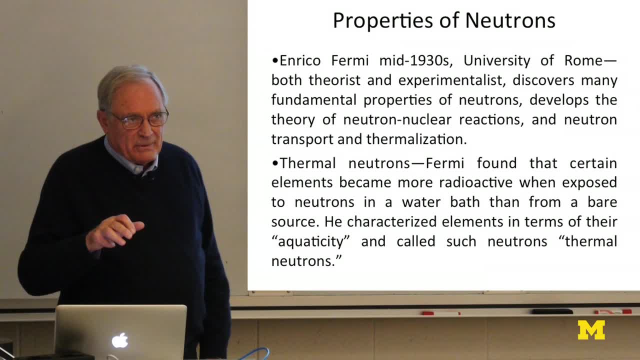 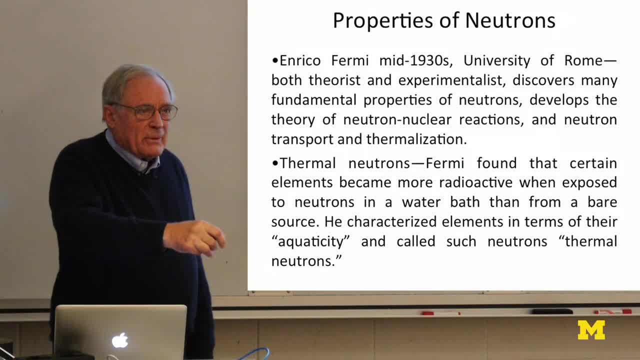 Neutrons In the Neutrons And he put his Is also toted up Neutrons for The source In What And then irradiated. Whatever ones He was testing Did became more radioactive. 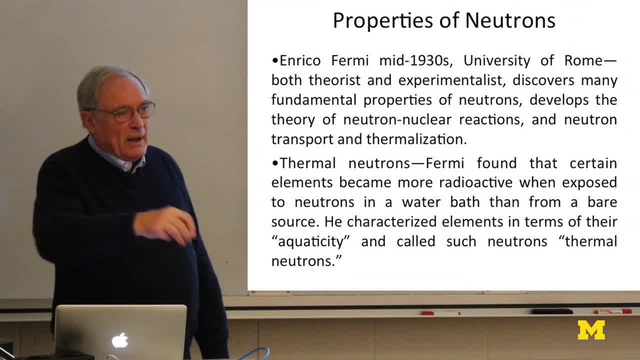 Then without The water present, And he characterized Different materials According to How much more The water cast The Things to become radioactive And he called that Phenomenon Aquaticity. You know We don't use that term. 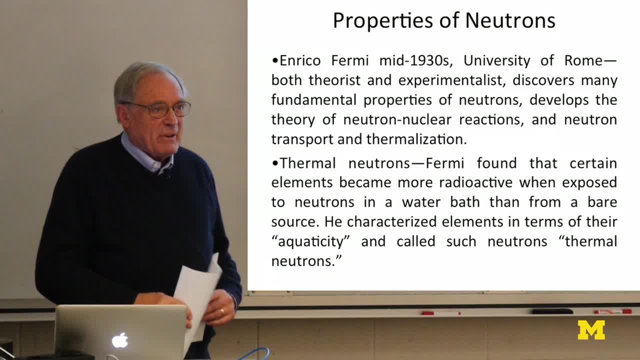 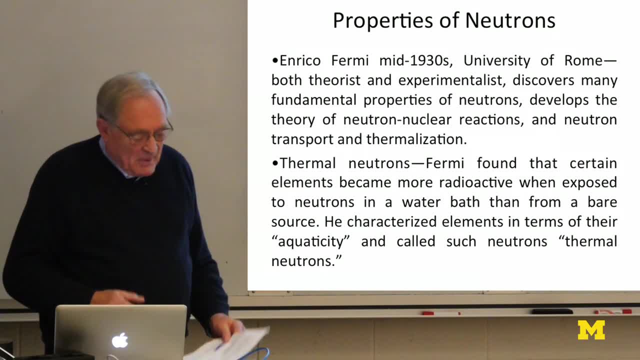 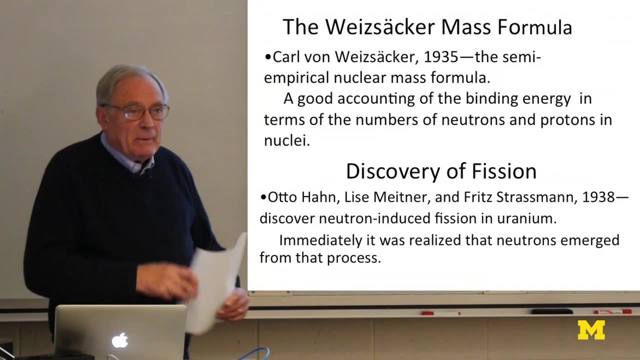 Anymore. Now we understand What was going: have a greater activation cross-section than fast neutrons. Sounds like it's falling off a log, but people didn't know that at the time. So then, Carl von Weizsäcker. 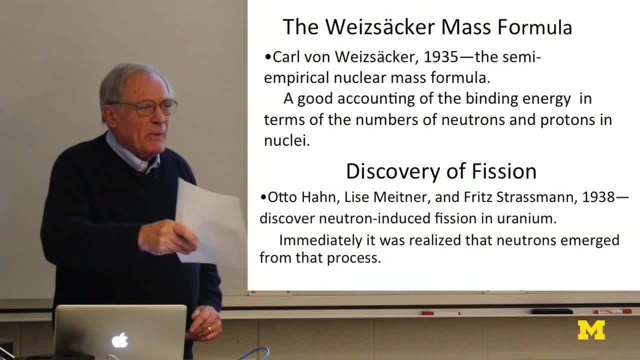 I don't know if people teach this at the time, but it's useful to know that teach this anymore. but it's useful to know that early on people understood the relationship between the number of neutrons and protons and the binding energies of the nuclei. 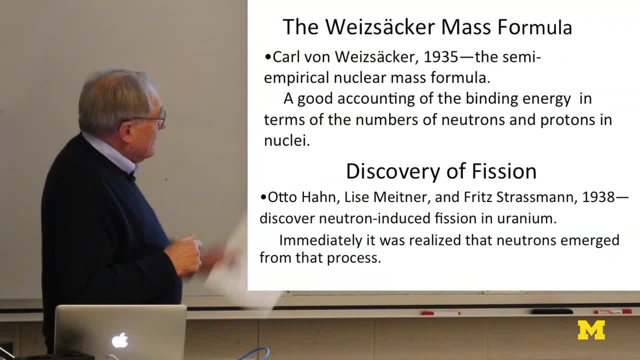 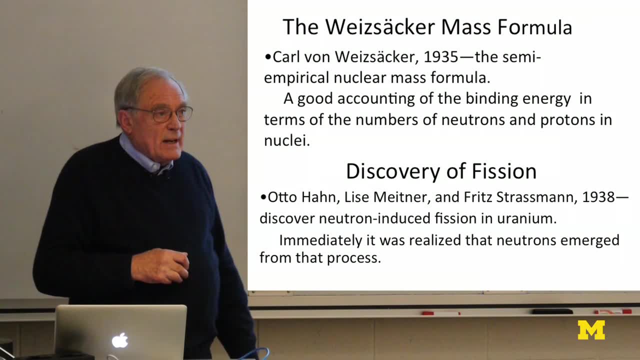 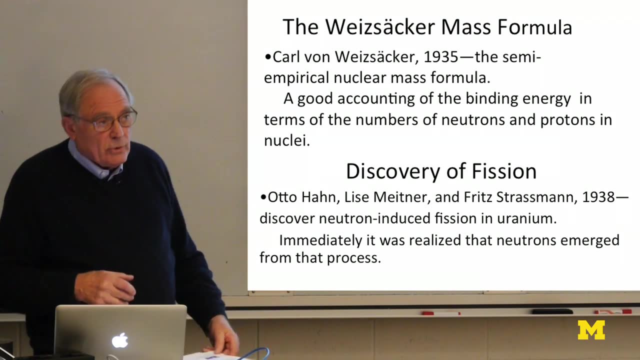 That had a bearing on the next discovery, that of fission. Otto Hahn, Lisa Meitner and Franz Strassmann were bombarding uranium with neutrons and they found additional radioactivity, and they concluded that this was due to. 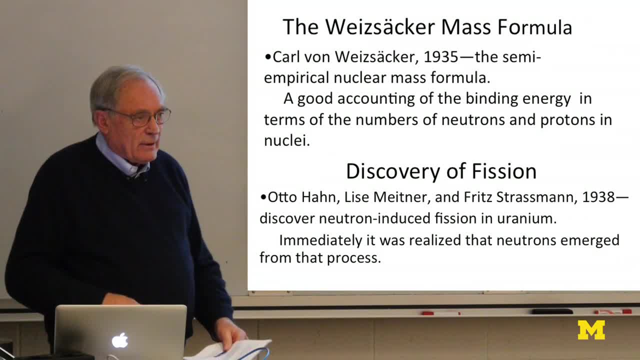 splitting of the atoms into lighter nuclei and they could identify because they knew about the activity of such fragments of barium and other lighter but half the mass of uranium. So they recognized these were fragments. but then if you say if these are fragments, 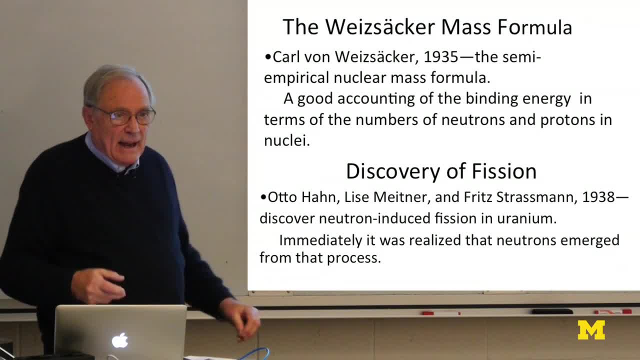 and uranium has so many neutrons in it and we break it in half and then each of these halves have way too many neutrons in it. so the reasoning was that there must be some neutrons giving off in the fission process. 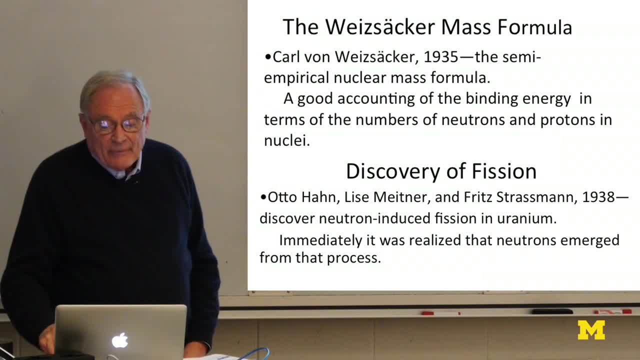 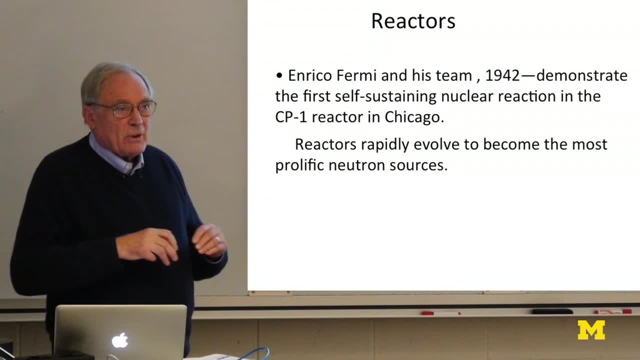 That's a very fertile idea, so to speak. And then Enrico Fermi and his team. there were others working on this, there were Germans working on this, and French as well, and Enrico Fermi, in 1942, was ahead of them all. 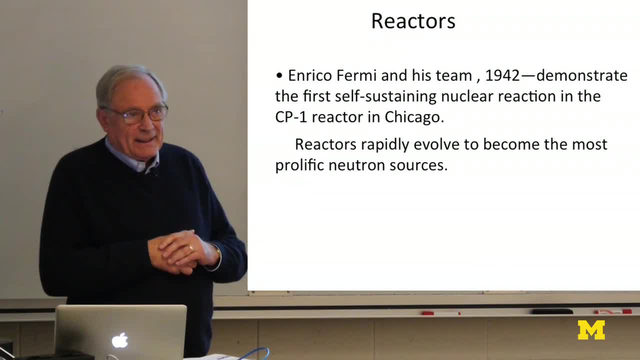 because he knew that carbon was a very good moderator And he built piles of graphite in order to test the graphite. he was looking for a source of graphite that didn't have neutron-absorbing impurities, And he found these. then he got ordered up a whole lot of these. 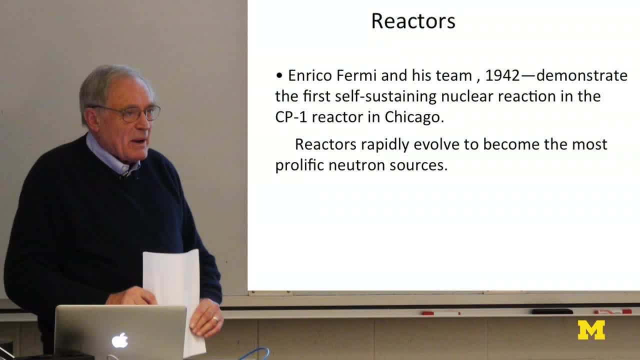 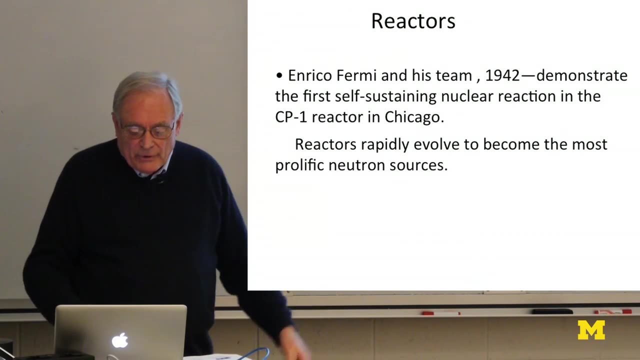 and they were working to build a self-sustaining reactor and he knew this. and they were working on this in the University of Chicago and by December 1942, after several smaller ones were built to show the principles- they built the first self-sustaining reactor. 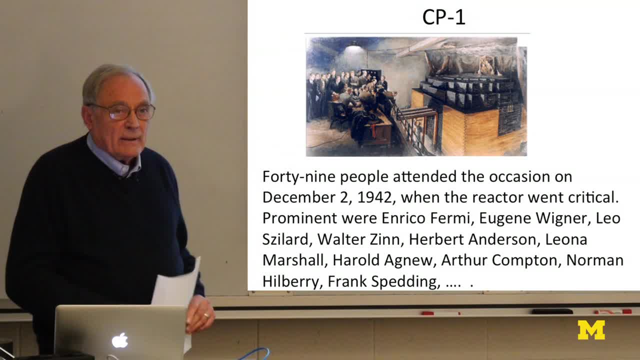 except for the one that was found in the swamp in Africa. that was critical three billion years ago or something. So this was the first man-made self-sustaining nuclear reaction, and there were about 49 people. the lights of the nuclear physics community. 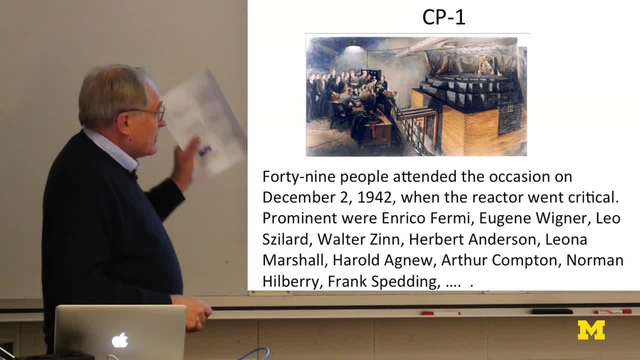 were there for the event. Like Enrico Fermi, he was the boss, Eugene Wigner, who was the brains who could design the first reactors, which he did. Leo Szilard, I think he patented the idea of a reactor. 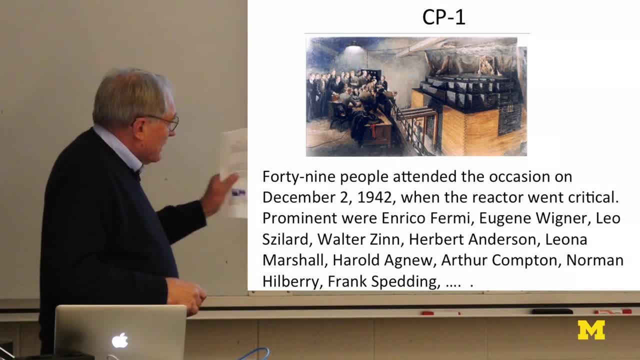 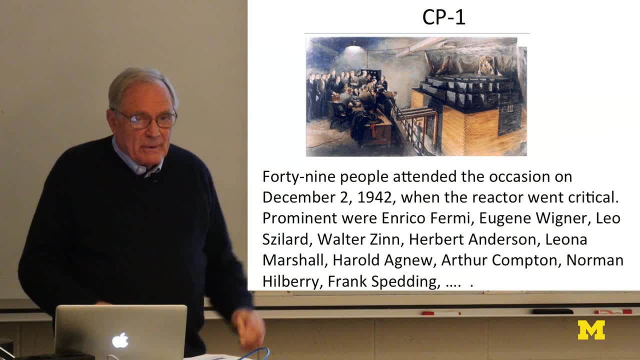 Walter Zinn, who was with Herb Anderson and others. they did some of the first experiments on neutrons using the beams from the first reactors. Now I'm gonna back up. History does not flow in a line. There are some lines that haven't converged yet. 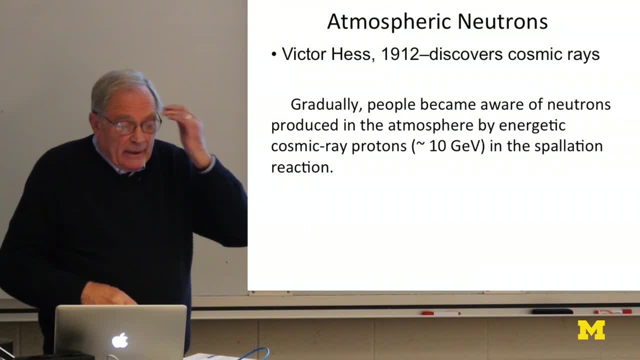 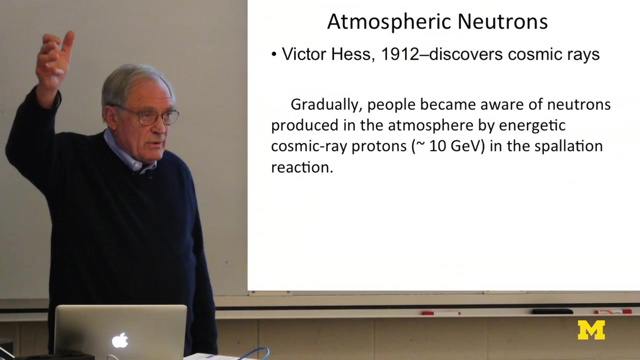 so here's one. In 1912, an Austrian physicist named Victor Hess discovered cosmic rays, and these are recognized due to very energetic protons, like 10 GeV protons, from the cosmos, not from the sun. 10 GeV protons penetrate the Earth's magnetic field. 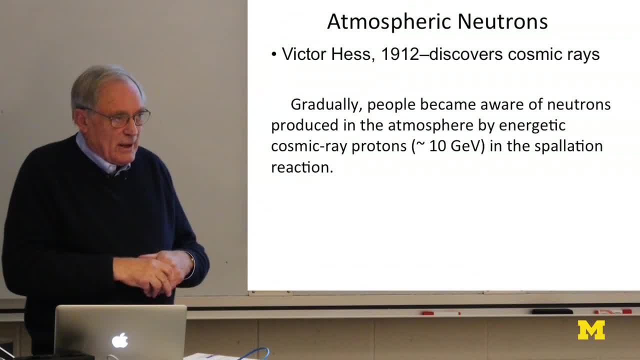 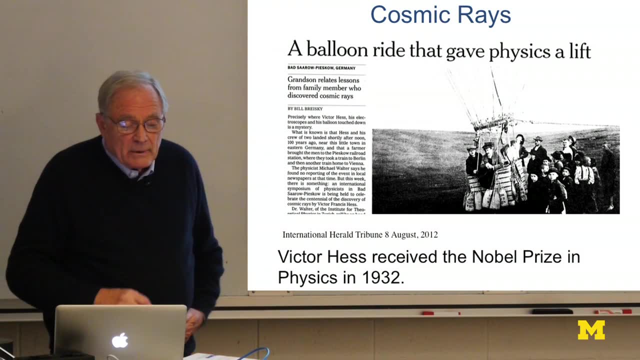 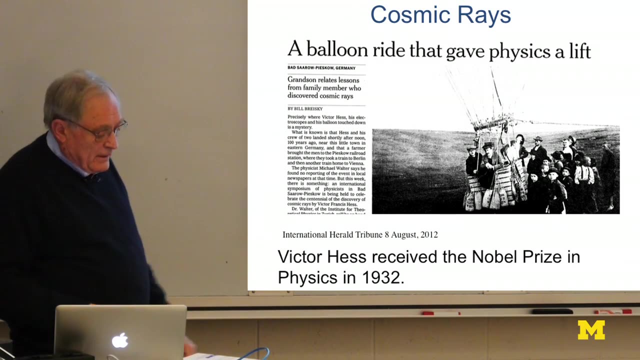 and these were the particles that Victor Hess discovered, And his discovery he made in a balloon flight with some colleagues in a nihilization chamber. He flew this balloon and measured the intensity of cosmic rays as a function of altitude. I have ridden in a balloon. 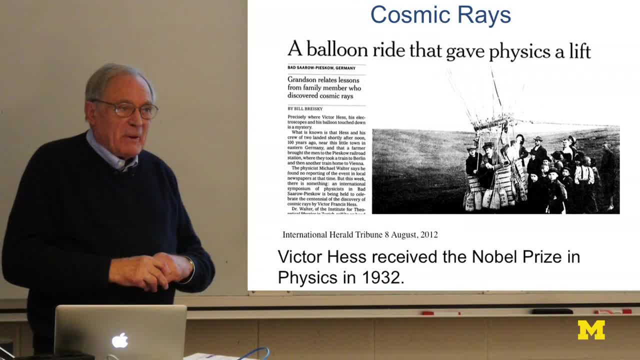 but I never thought to carry a cosmic ray detector with me. But anyway, turns out that the intensity of cosmic rays increases the higher you go, And he discovered that. So there are neutrons in the atmosphere and that was a matter of 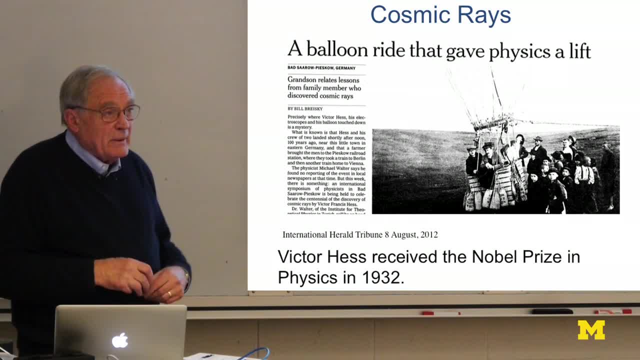 an observation of some fascination. It provided you knew they were there- 10 GeV protons which are energetic enough to do nuclear physics, And that was the way you did this. in those days You didn't have accelerators to produce. 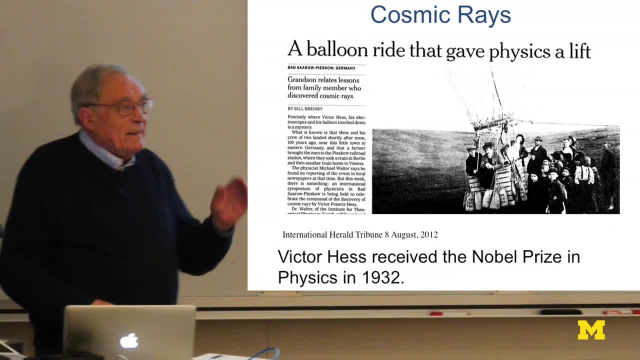 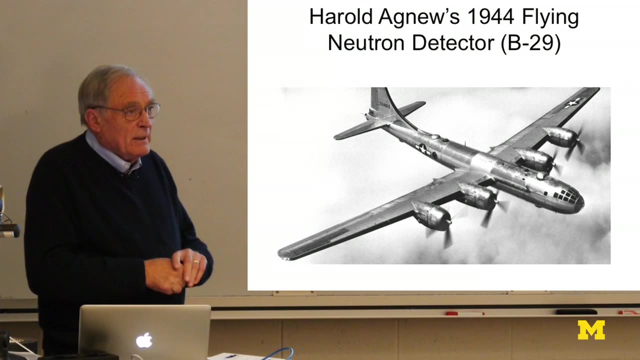 sufficiently energetic protons. but people were still doing or making observations of nuclear physics phenomena using cosmic rays. So it was known that they were there and it became a matter of curiosity what the, how much the neutron component was. what was the? how did the neutron component 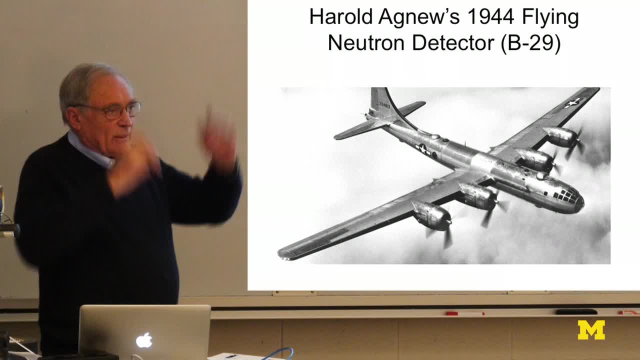 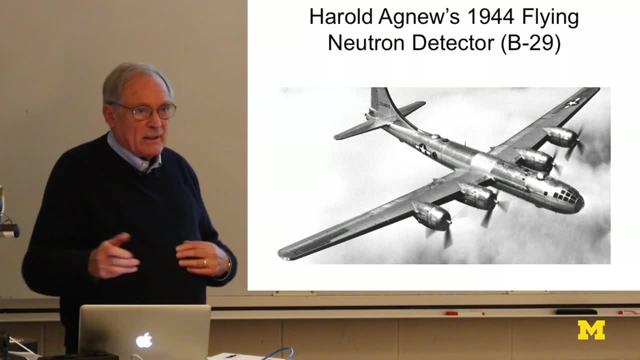 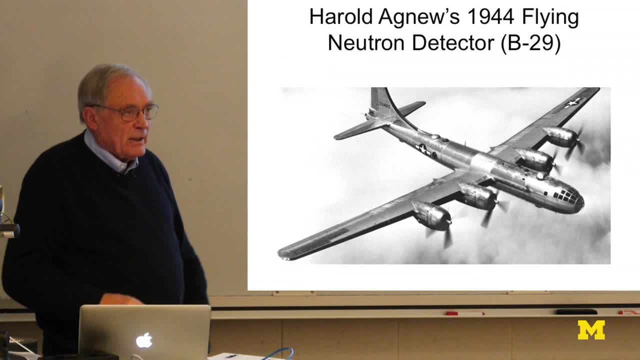 Anyway, he was a young man in the Manhattan Project and he borrowed a B-29 bomber, put neutron detectors in it and flew them over. you know where he was because he reported data from 7,000 feet up to about 40,000 feet. 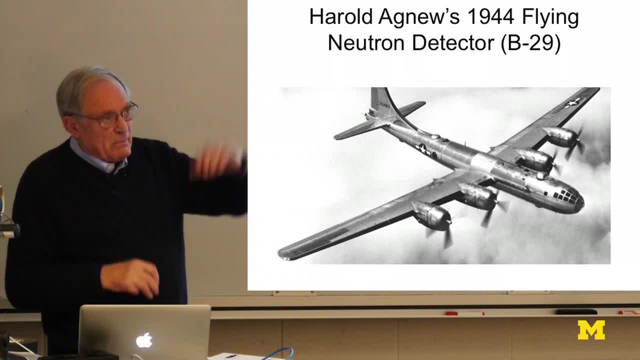 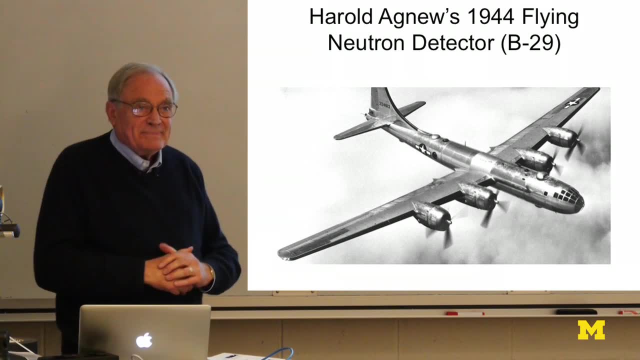 Now the 40,, the 7,000, 40,000 feet's, the sort of more operating altitude of B-29.. The 7,000 feet happens to be the altitude of Los Alamos. That's where he worked. So people then knew that this. 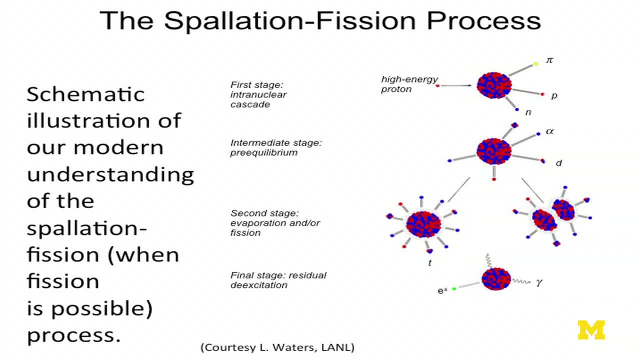 neutrons were produced by a process called spallation, due to high energy protons interacting with nuclei, and this illustration shows a proton hits a nucleus, collides with one of the nucleons. nucleons distribute the energy inside the nucleus. knock out a few light particles and in between, the first like 10 to the minus 20th seconds and the next 10 to the minus 15th seconds. all the energy is uniformly distributed in the nucleus and it gives off particles. The alpha particles, deuterons, neutrons and even some lighter stuff. heavier stuff like carbon and nitrogen, evaporates in the process of cooling off. So you get all these particles in the process of cooling off and losing the energy and the main decay product. of this hot nucleus is neutrons, because they're charge-less and are bound with less energy, and so you're left with a bunch of neutrons from evaporation, and then you're left with, when you can't evaporate, neutrons anymore. 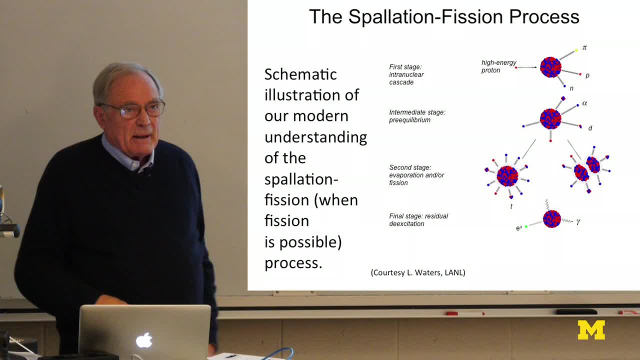 you have a radioactive nucleus, maybe decays with the emission of beta particles and gamma rays. Otherwise, sometimes it's got a fission and what happens from there on is like we all understand about fission. You have just a pair of lighter fragments which evaporate neutrons. So a lot was known about this, from Harold Agnew's flight, from people flying in balloons and measuring the neutron intensity as a function of altitude. And here's Enrico Fermi's summary of all that data that was well known in the 1940s. 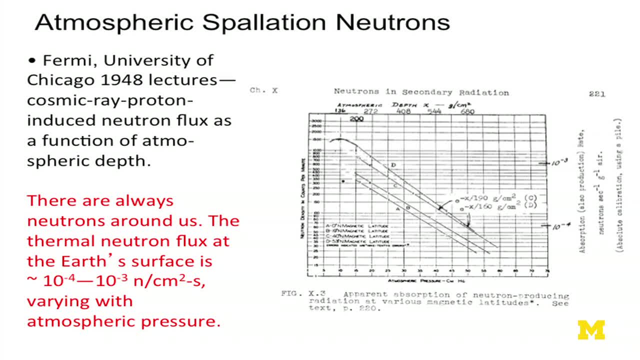 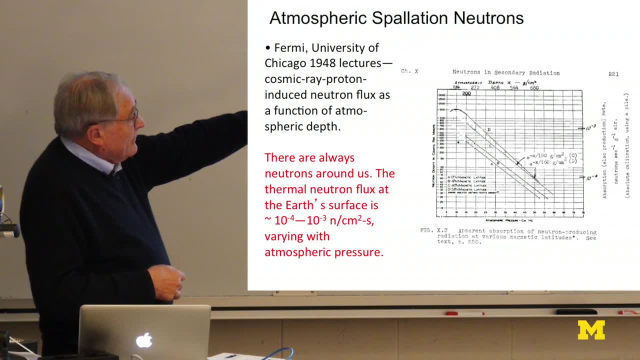 This is in his book of lectures from his lectures at the University of Chicago in the 1940s. So the numerical values and the variation of the neutron flux as a function of altitude was known in the 1940s. And not only was it known. I want you to know what I've written in red. 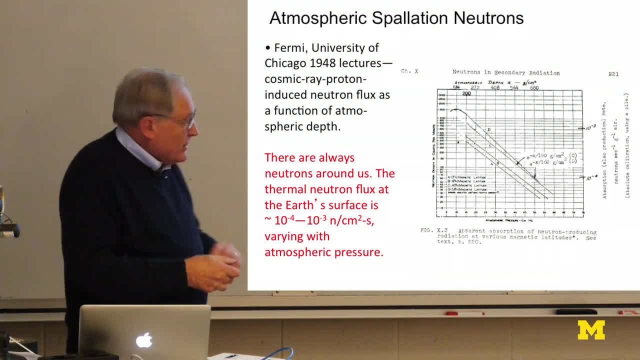 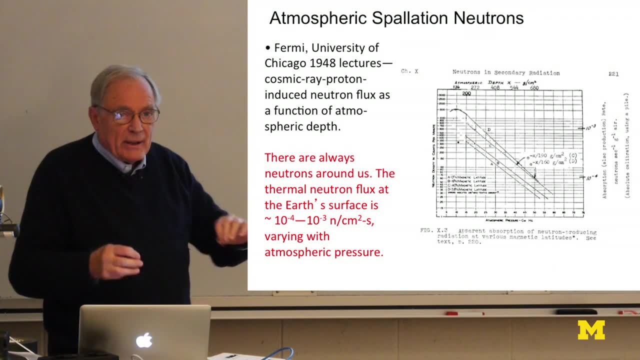 that you always have a flux of neutrons around you. It is around 10 to the minus fourth or 10 to the minus third neutrons per square meter per second, which is something like one or ten neutrons per square meter per second. 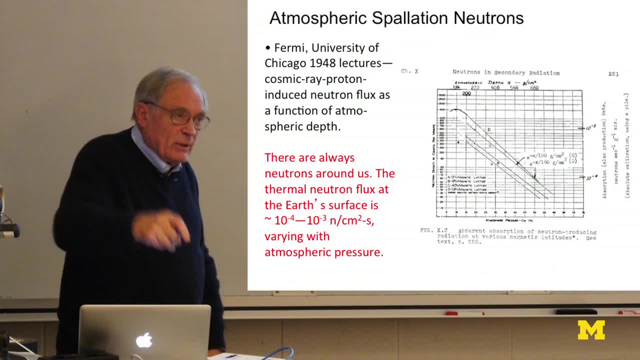 And if you have a meter square detector and you're testing it, if you see neutrons, there's nothing wrong. That's the cosmic ray background. But if you have an electrochemical cell and are looking for cold neutrons, you will see neutrons. you will see neutrons, but they're not from the electrochemical cell. 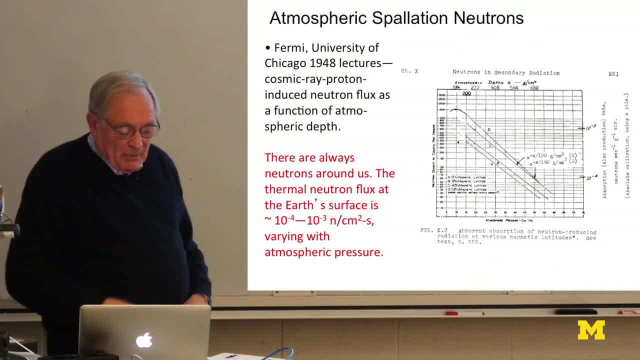 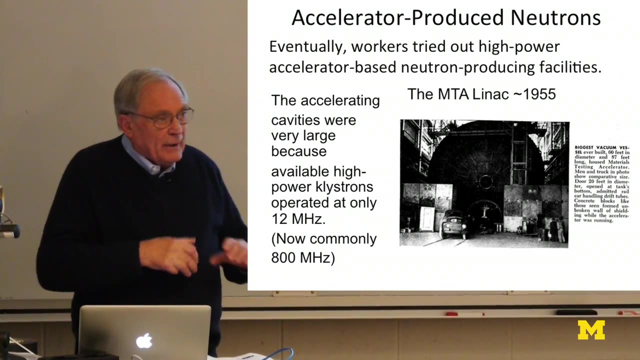 I mean, a lot of people made that mistake in the old days. But the data that people should have been aware of is already present in Enrico Fermi's book. Well, people knew about it. People knew about making neutrons with particle accelerators. 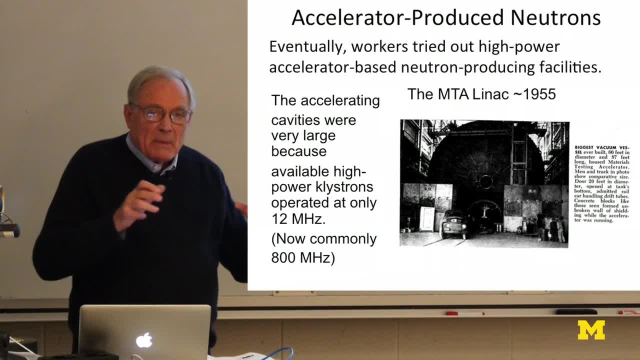 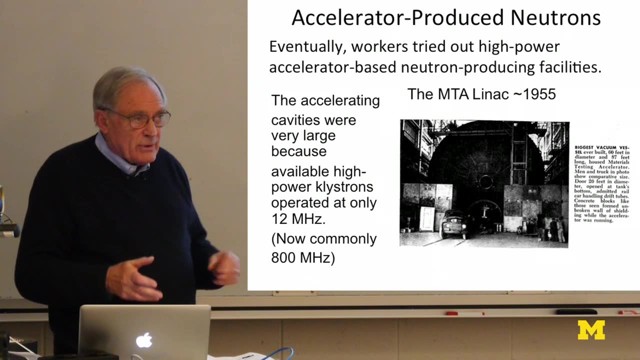 And one of the big efforts of the Manhattan Project was to produce reactors to breed plutonium, to make atomic bombs. So a big effort to make plutonium. And one of them was the reactors that Fermi and Wigner designed. They were the production reactors at Hanford. 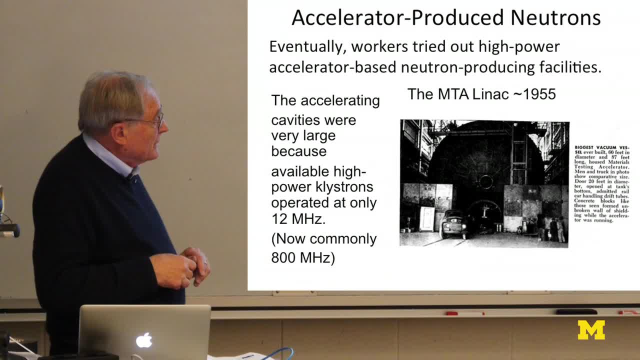 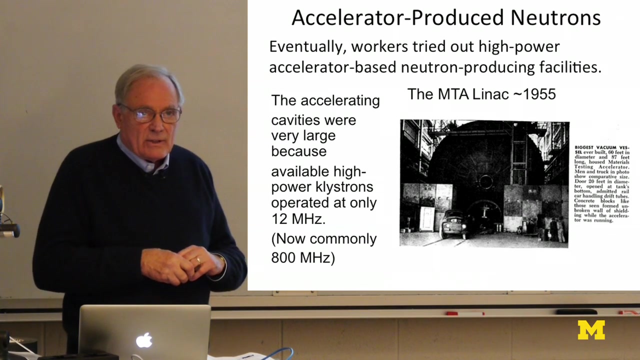 But on the other side was this effort to use accelerators. So here's a picture of one of the early accelerators that was built in the 1950s. Actually it was called the Materials Testing Accelerator, the MTA. The project was declassified in 1955. 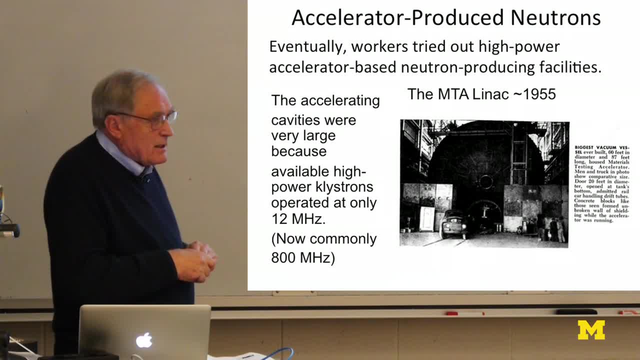 So the MTA was Materials Testing Accelerator, except it had nothing at all to do with materials testing. They were going to use this accelerator to breed plutonium. So this was not a bad- not technically a bad- idea, But in those days the klystrons that you would need to build the accelerator only would run at about 12 megahertz and the accelerating cavities were, of course. 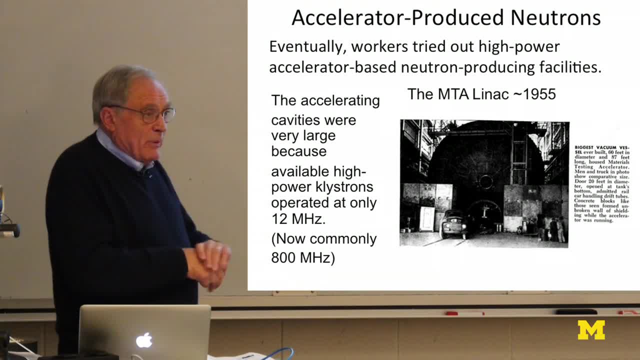 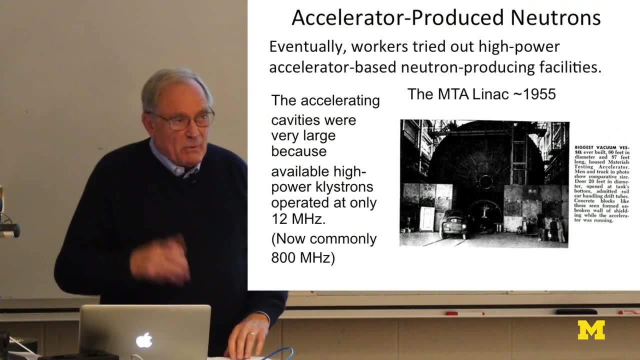 correspondingly huge, And this is a picture of the vacuum chamber they built for the MTA accelerator. It was abandoned in 1955 because people discovered deposits of uranium in Canada, But it wasn't a materials testing device. However, it was one of the very first neutron-producing devices. 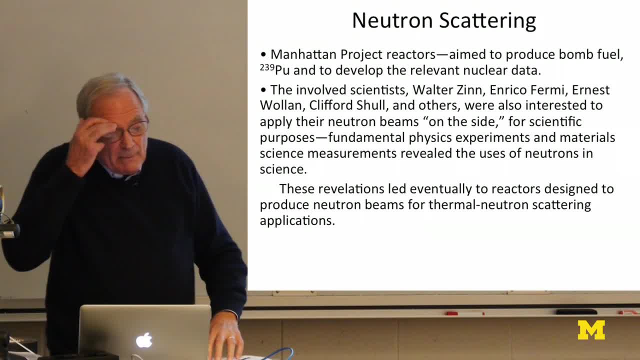 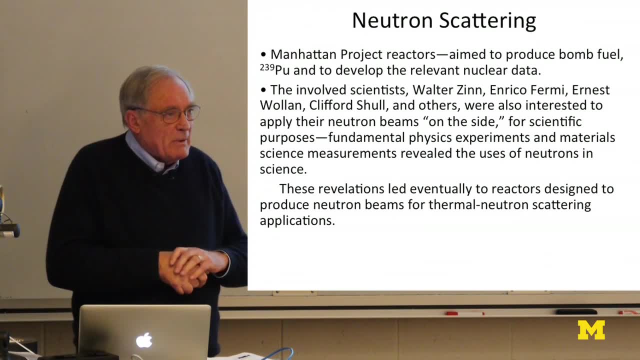 So back to the Manhattan Project. The people working on there were building reactors And they finally built powerful enough to make neutron beams to do experiments with And of course, these were very useful to learn the properties of some of the materials in the reactors that they were trying to build. 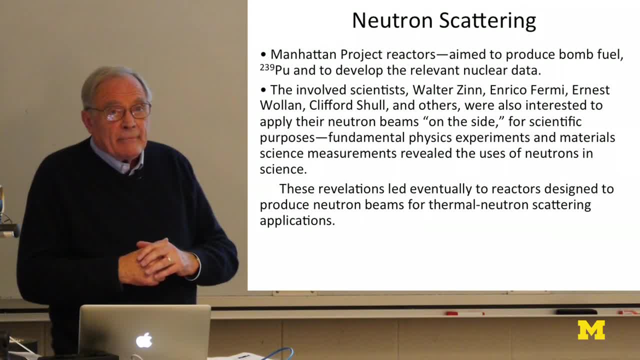 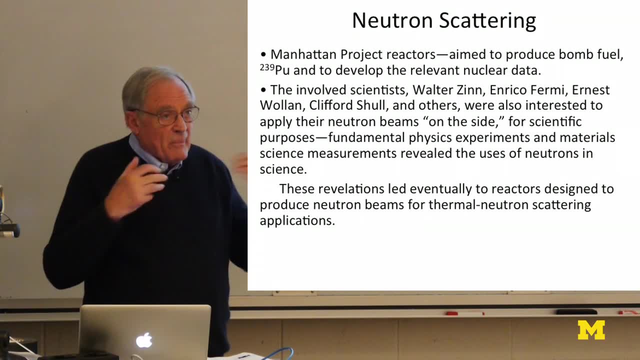 So it was all part of that same effort. But the scientists were not satisfied just to do this kind of civic duty. They had neutron beams- Delicious idea, Let's see what I can do with the neutron beams for my science. And they did scientific experiments. 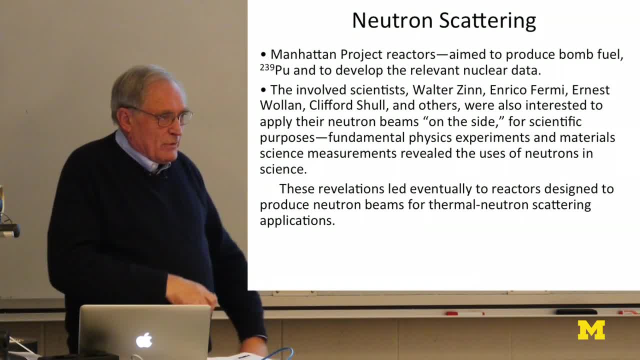 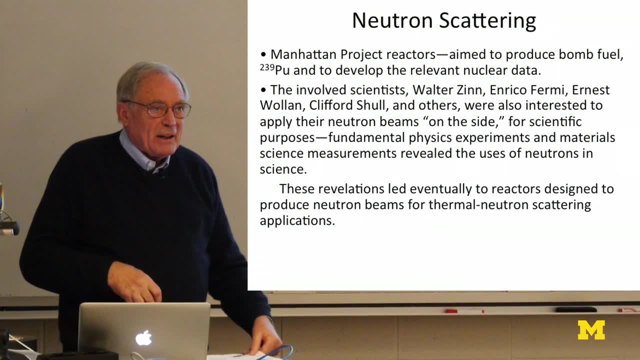 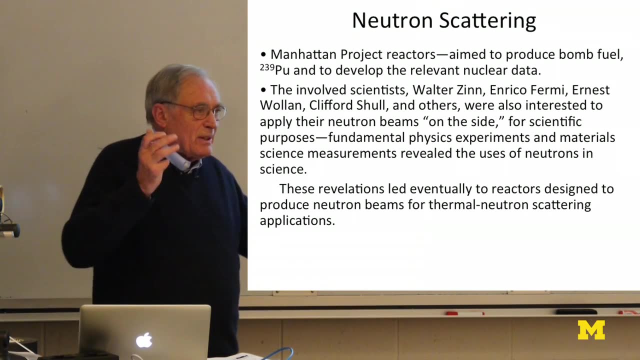 Like they demonstrated that neutrons would reflect from surfaces like a mirror And they could measure the scattering length of the nuclei, which were important to understand if you were going to go any further. And they did some diffraction experiments that showed you could actually diffract from hydrogen. 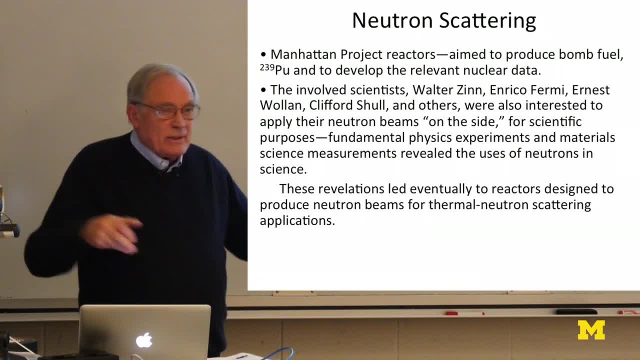 OK, I'm sorry- in solid materials, which x-rays don't do. so they look for openings for these applications And this grew into a fairly big effort of neutron scattering as a method of doing material science research. That's where I sort of 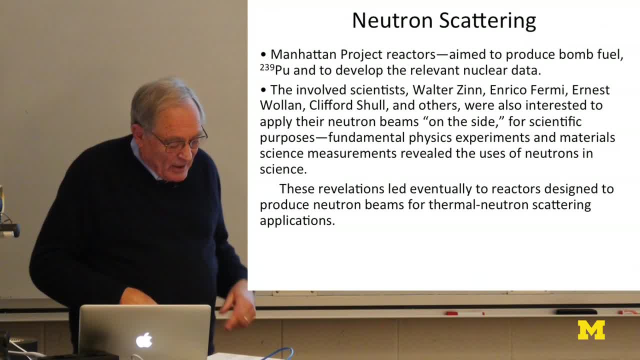 my own interest was kindled at that point. So what kind of reactors, You might say. well, we have 104 power reactors. why don't we have neutron beams from them? First of all, they are not high flux. They are big and low flux. 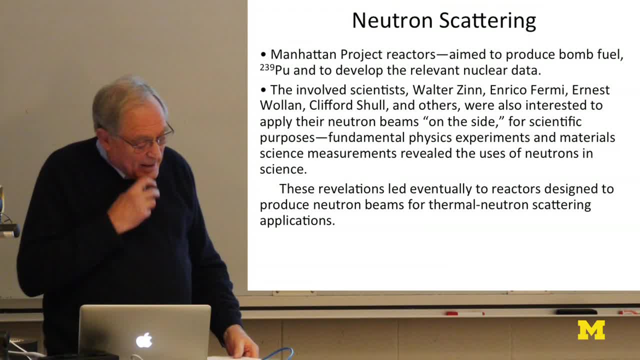 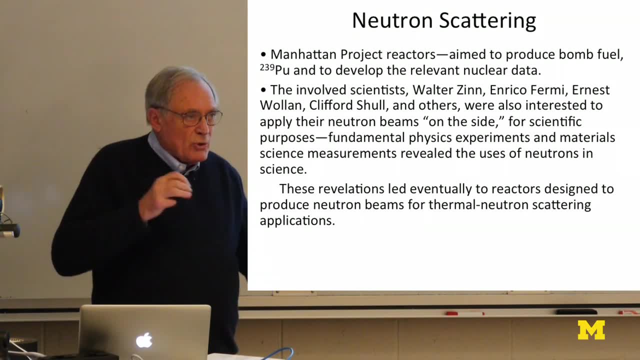 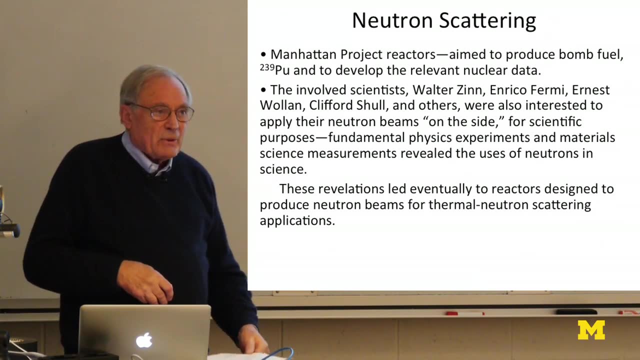 and they meant for the fuel to last a long time. On the other hand, research reactors to produce intense neutron beams are designed for high flux, maybe short fuel lifetimes, but they are very difficult to produce, They're dense and small and they're completely different animals. 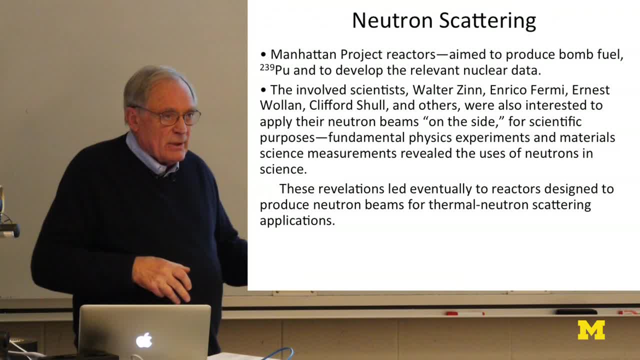 Furthermore, neutron beam reactors. research reactors have holes for the neutron beams. The story is that Dick Cheverton, who designed the high flux isotope reactor, somebody said, Cheverton, I want neutron beam holes in my reactor. And he said what? 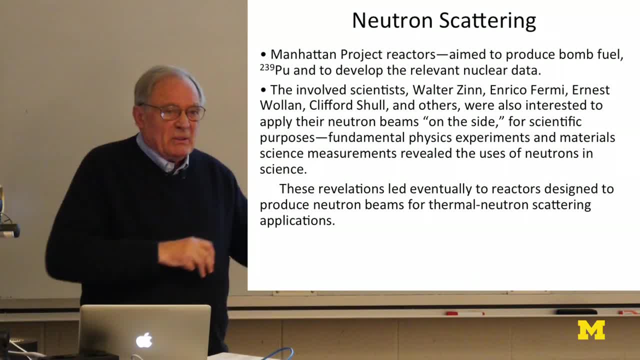 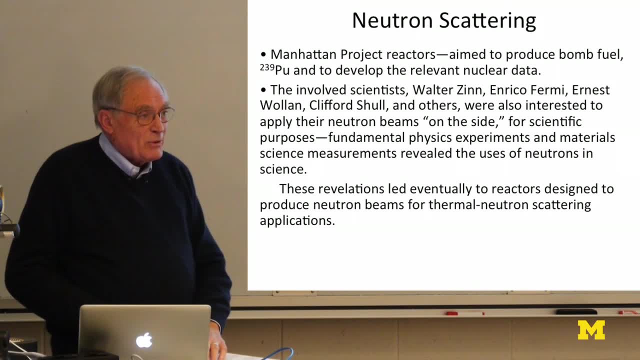 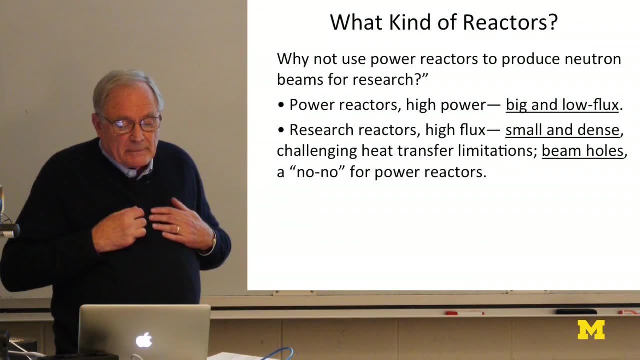 Holes in my reactor? No, sir. Well, eventually they did put beam holes in the high flux reactor and it still exists today. But power reactors are not the place for beam holes. I guess I didn't have this picture up at the time. 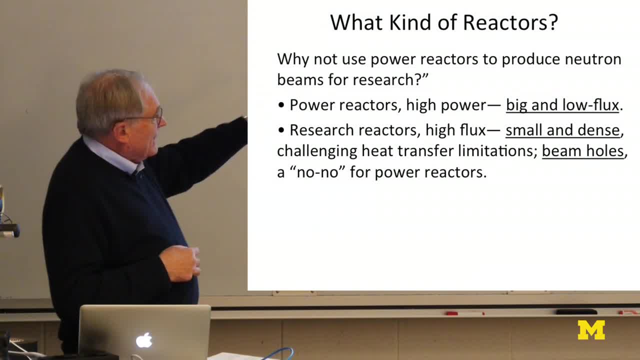 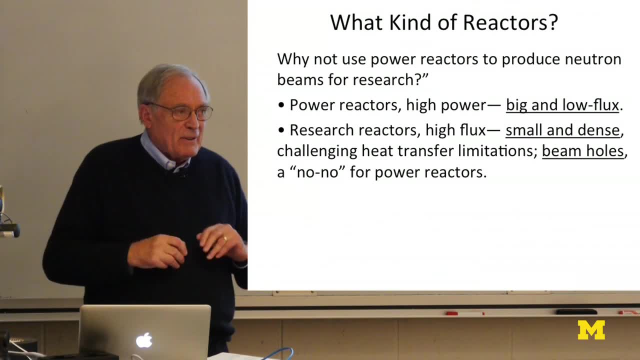 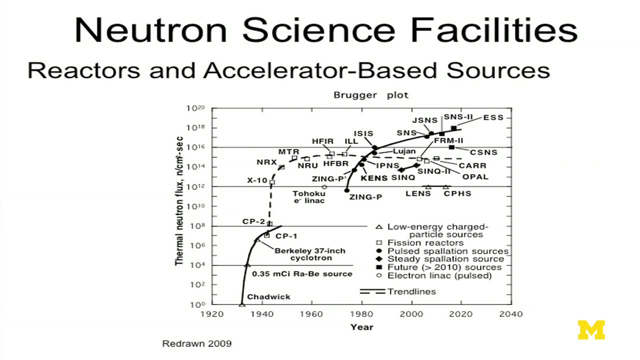 So power reactors are big and low flux. Research reactors are small and dense and high flux and they push heat transfer limits. So that's where the game is: in designing high flux neutron sources to beat the heat transfer limits. And here's where we've gone. From Chadwick, with one neutron per square centimeter. second neutron source and higher intensity from radioactive sources. then a neutron source based on a 37 inch cyclotron, big enough to accelerate to some tens of MEV and actually produce some neutrons. 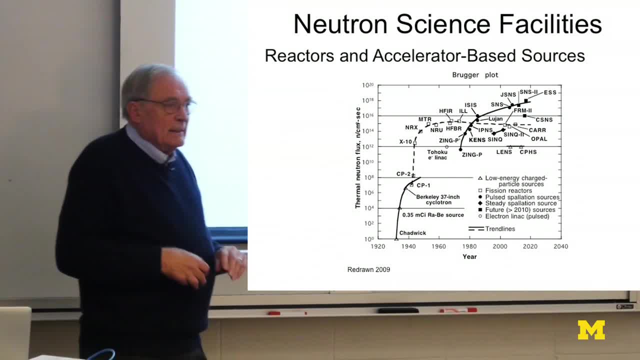 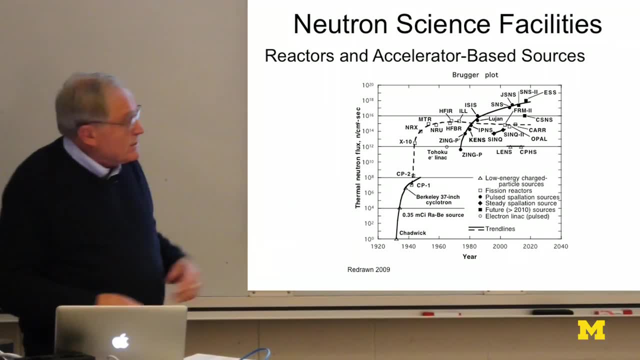 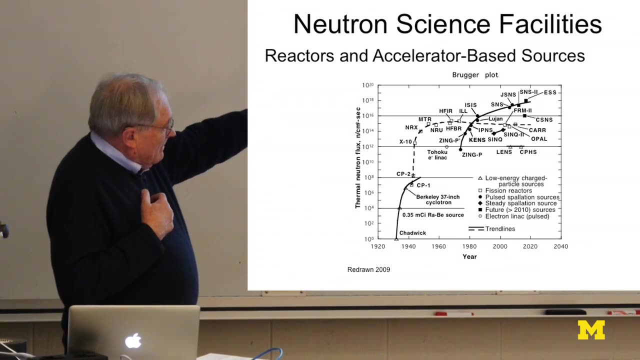 And then CP1, the first reactor had a rather low flux, But the technology was there then to go up to much higher fluxes And as years passed, people built more and more powerful reactors and higher flux reactors, until they reached about a 10 to the 15th neutron per square centimeter second. 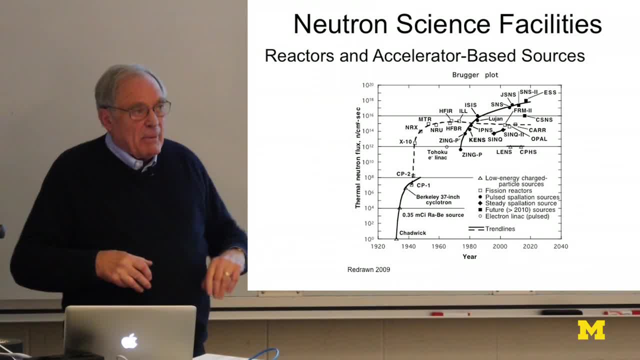 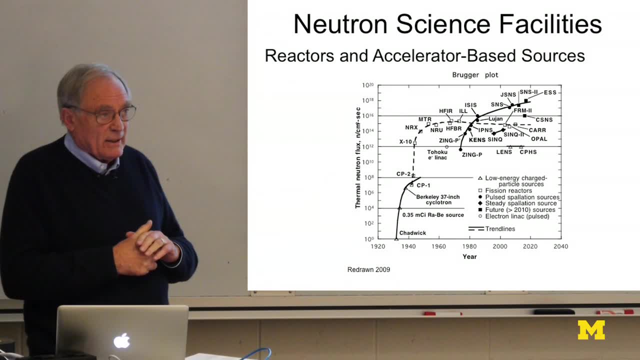 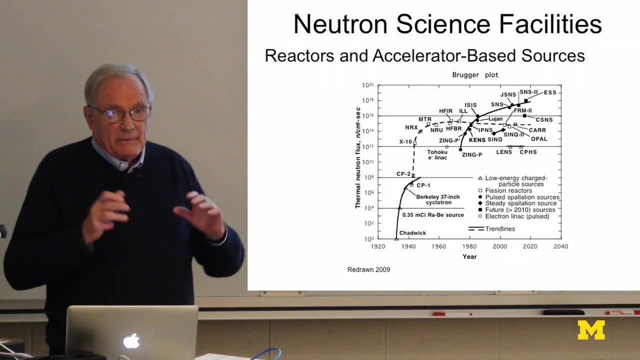 in reactors that have about 50 or 100 megawatts of power And that's the limit, And not building any reactors that can produce much higher flux. There was a long term effort at Oak Ridge to build a what was it called. 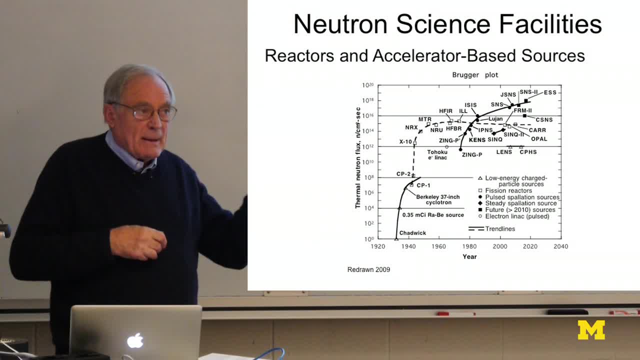 Advanced neutron source with a neutron flux about three times higher than ILL. They worked on this for 10 years and the project became more and more costly and more and more doubtful and they dropped the project in 1995.. That was the end of the line. 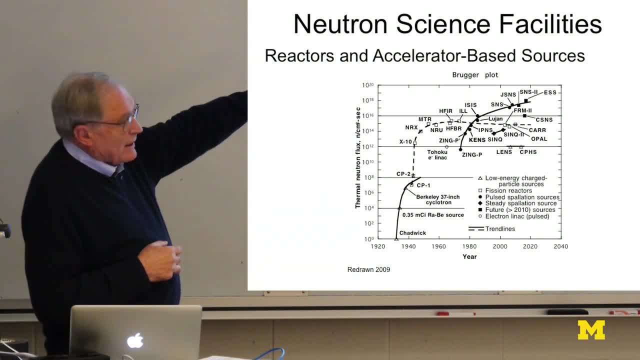 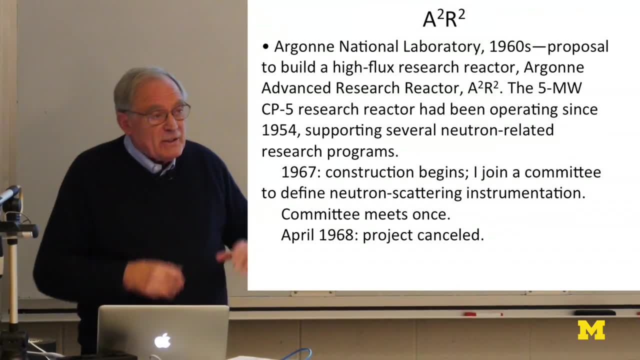 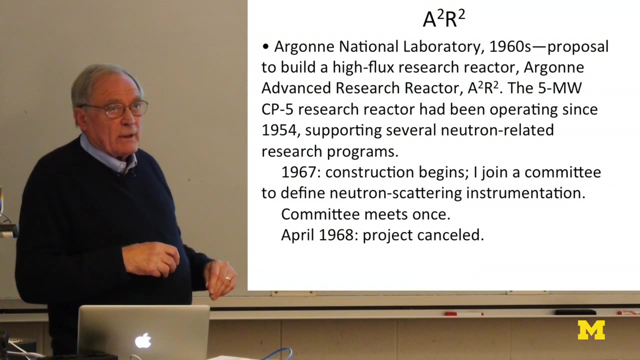 So you don't go much beyond 10 to the 15th neutrons per square centimeter second with reactors. And then there's a question of how can you do better In that same era, regardless of having beaten up against the heat transfer limits, Argonne wanted to join the game. 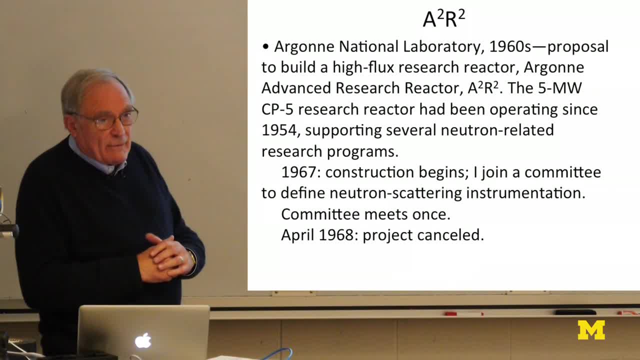 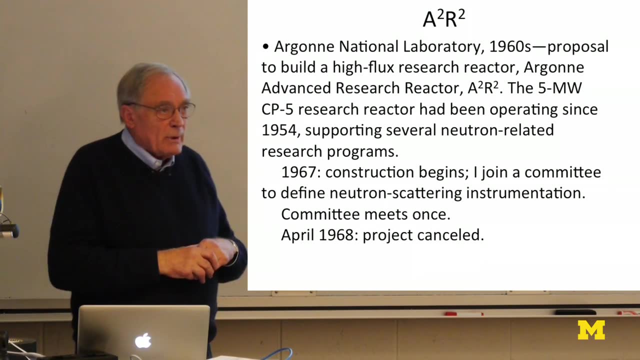 That was along with the HIFR reactor that was being built HIFLUX isotope reactor at Oak Ridge. They proposed the Argonne Advanced Research Reactor. A squared, R squared, And that had some funding. Meanwhile Argonne had been running neutron research programs. 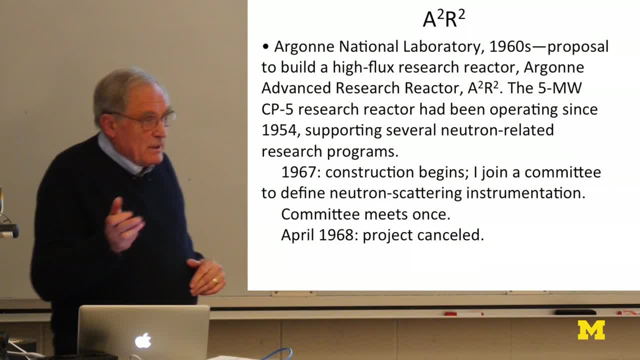 at the five megawatt CP5 reactor. So there was a big interest in Argonne And construction on A squared R squared began in 1967.. I was asked to join a committee on instrumentation for neutron scattering at the A squared R squared. 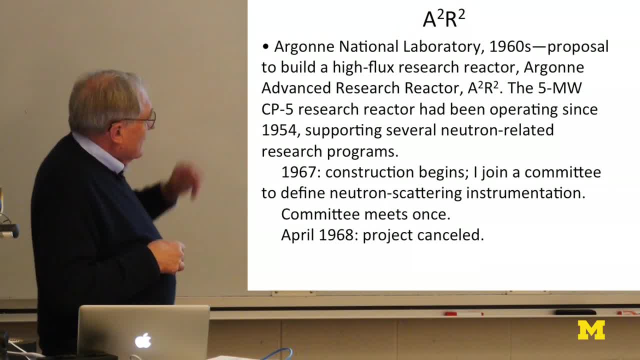 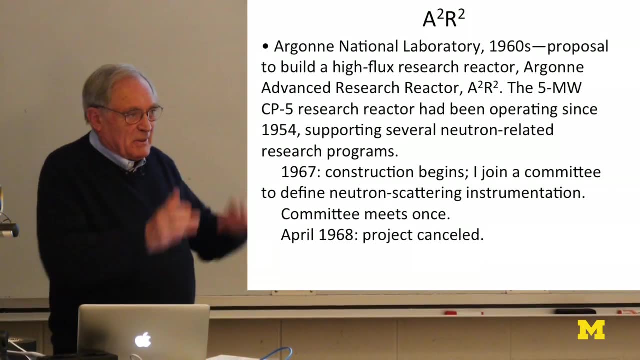 So we met in January, I think it was to define neutron scattering instruments for A squared, R squared. Then within weeks the project was canceled. Concrete that had been poured in the ground is still there. Project was canceled in April of 1968.. 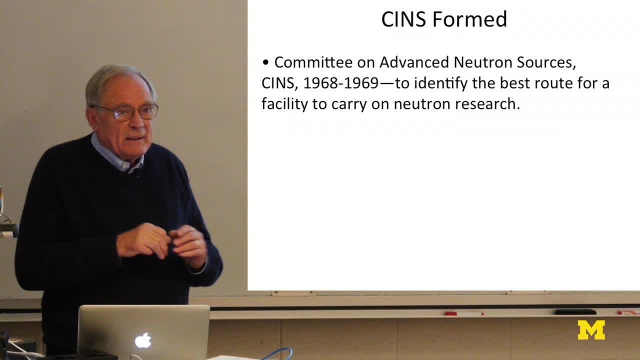 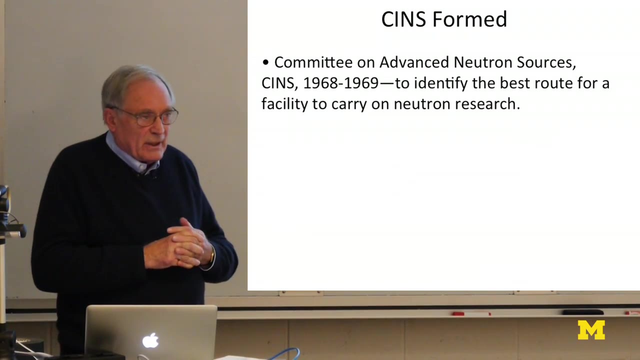 So Argonne had was interested in neutrons and they thought we'll see if we can continue And formed a committee on advanced neutron sources or a committee on intense neutron sources And that committee met from 1968 until 1969. 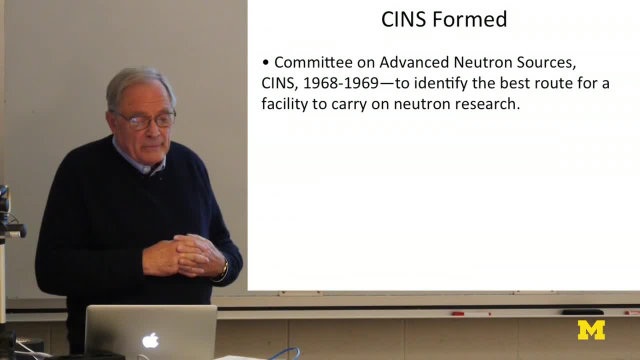 And they asked me to join that committee. Mostly people doing neutron scattering or reactor design or fast neutron cross-section measurements and things like that. So a lot of neutron people, a lot of reactor people, a lot of accelerator people. So the Committee on Intense Neutron Sources. 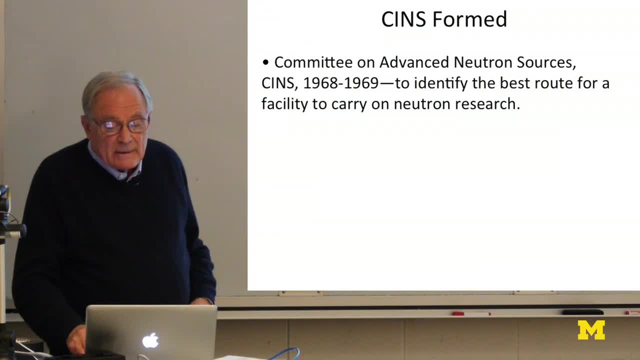 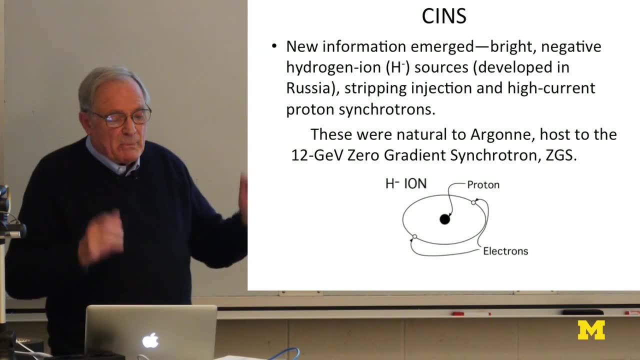 began meeting in mid-1968. And I went there to meet with them And new information. they uncovered new information. What was important, One of the members of the committee was an accelerator physicist who brought back knowledge of a bright negative hydrogen ion source. 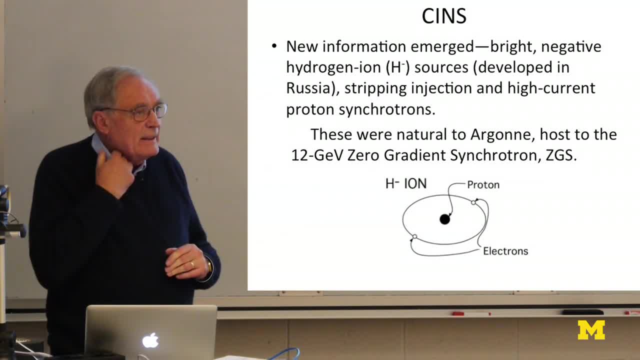 Had been developed in Russia, And the idea was to use this to inject higher currents into a synchrotron ring. You could do this instead of just running protons, in which that you would say, I'll run them in and I'll deflect them at the magnetic field. 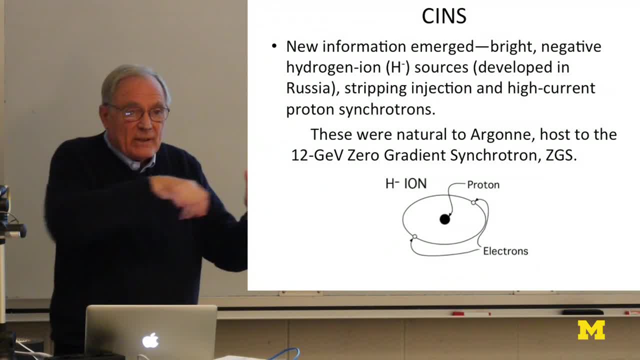 and put them in the orbit, And then I'll put some more in the next orbit. Well, this is limited by Liouville's theorem. You can't do that more than so-and-so. A space charge limit is an intrinsic feature of an accelerator, and you can't beat it by using reversible methods. 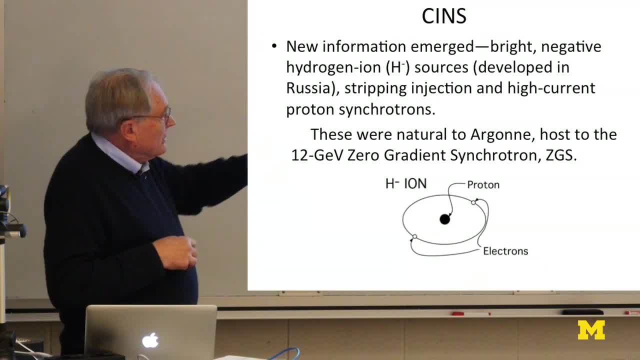 But with negative hydrogen ions like are shown here. the proton has two electrons and it's a sort of quasi-stable thing. but you can have a source of these- and that was what was discovered from Russian experience- and pass them through a thin like a few microns thick of carbon foil or something. 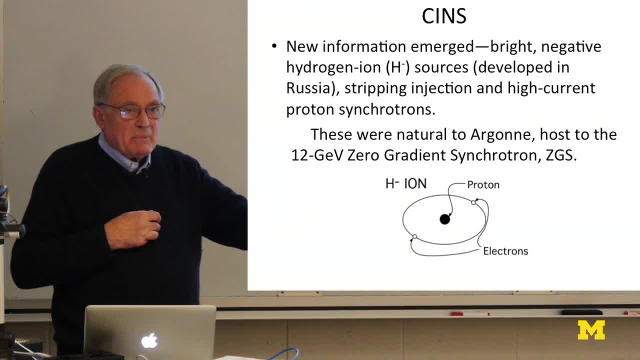 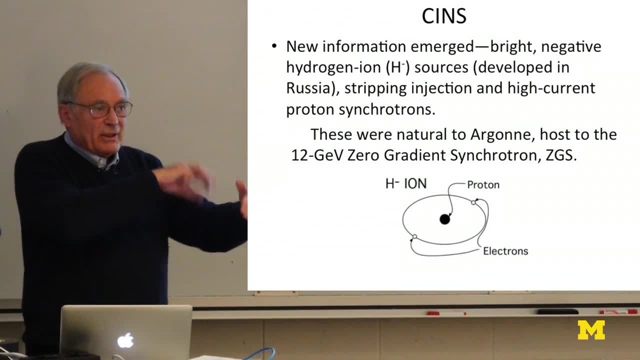 the electrons come off and a negative hydrogen ion becomes a proton And it would circulate in a ring like a proton, But it went in as a negative hydrogen ion, so it's bending this way. Protons that are already circulating are bending this way. 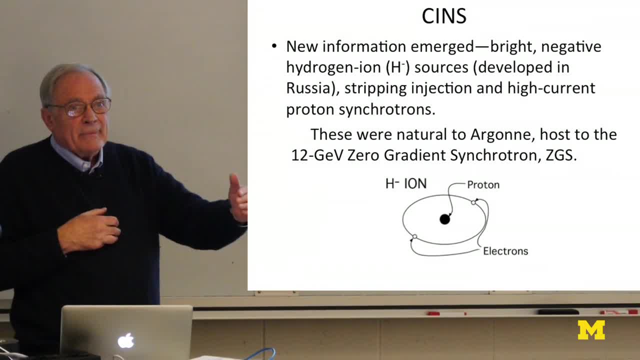 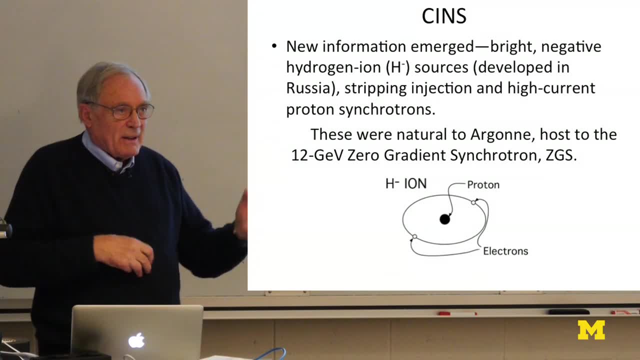 They go through the foil many times, and foil doesn't do much to them, So you can keep piling them on. and this is not a violation of Liouville's theorem, because the process of stripping is an irreversible process. So this was the idea. 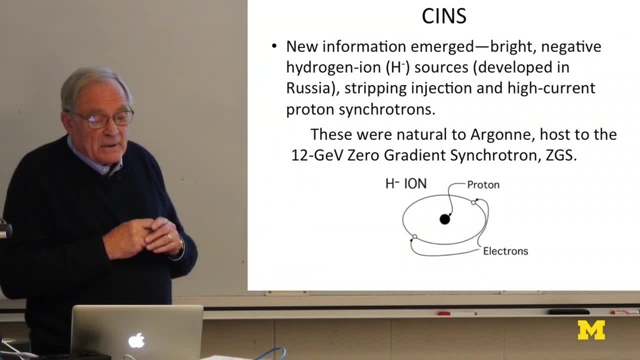 And the committee just found it natural to apply this To increase the intensity of protons in the zero-gradient synchrotron, which is the big machine of the day that was working at Argonne lab. So the information about stripping injection and negative hydrogen ion development. 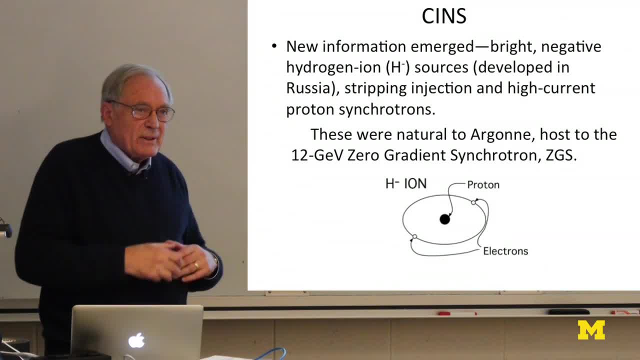 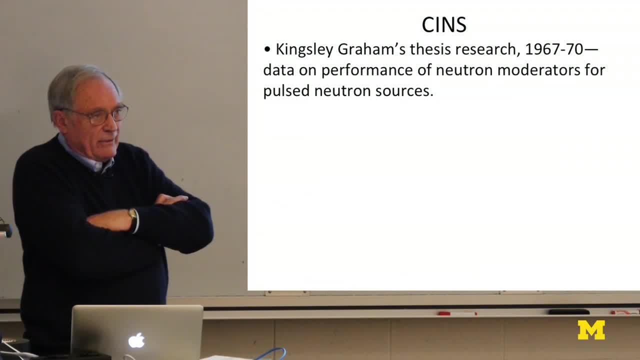 was out there and was one of the ingredients that the committee on intense neutron sources had to deal with. Then there was another component of stuff. I've been working with Kingsley Graham, who is here now, to do measurements on moderators, So you needed to know how neutrons slow down. 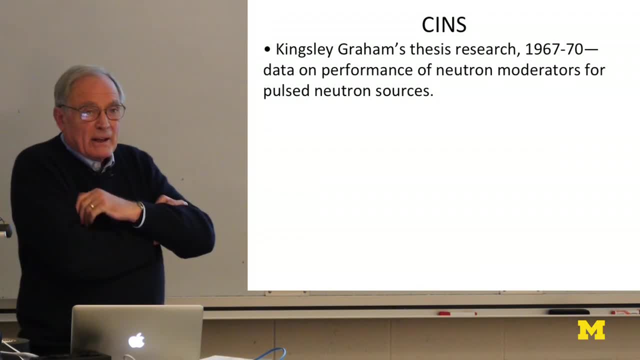 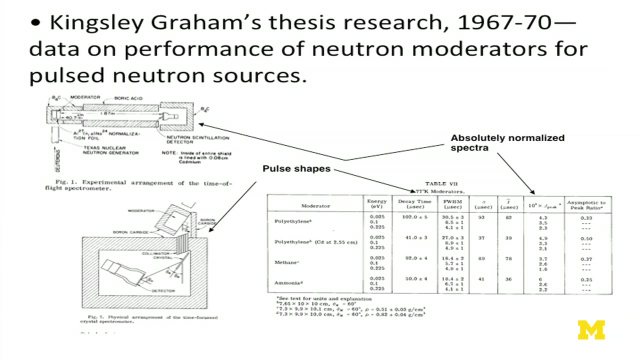 in a productive and reliable way in order to design anything But Kingsley's measurements showed not only what the spectra look like, but what is the shape and width of the pulses that you would get, And with this information you could then design a moderator. 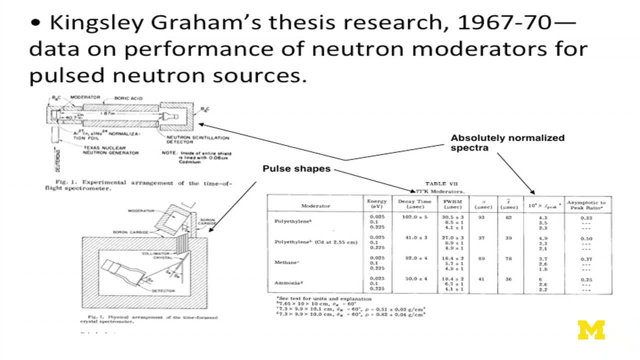 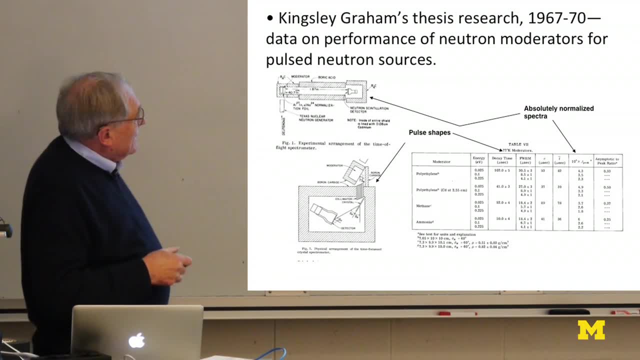 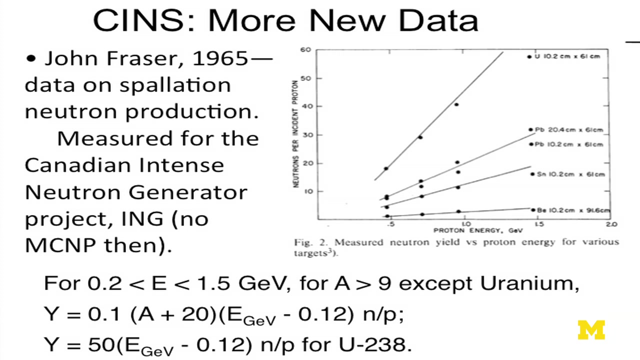 So Kingsley Graham's measurements made that possible. They gave information from a pulse source moderator. These are the two devices that Kingsley used And it was central to being able to conceive this next step. There had been work in in Canada to develop an intense neutron generator called ING. 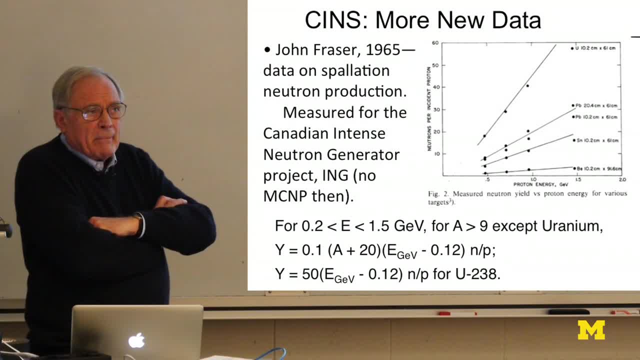 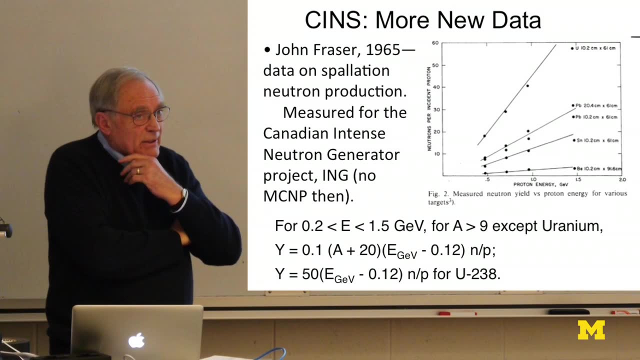 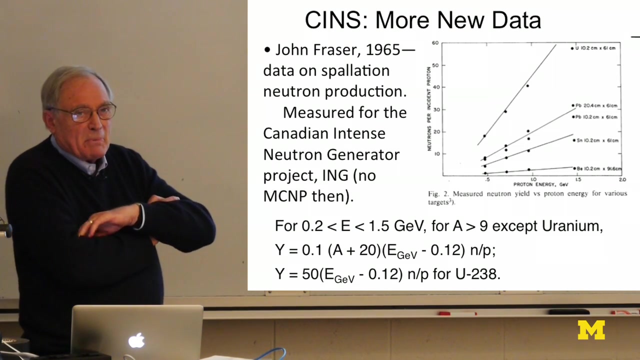 They wanted to produce a one megawatt proton beam based on 60 MeV LINAC a mile long. So that was the idea. And to support that design, John Fraser and a team of others who worked at the Cosmotron to measure the number of neutrons produced by protons. 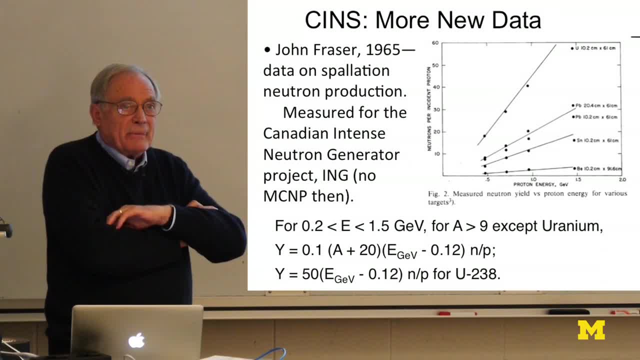 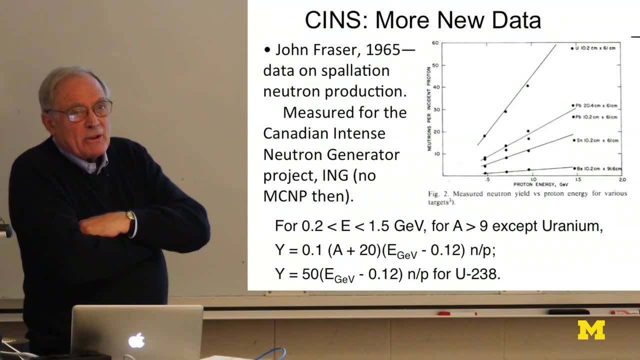 People knew that neutrons were produced by protons, but the numbers weren't absolutely known. So Fraser went about measuring absolute measure. So he measured what I've showed in this chart: How many neutrons per proton as a function of proton energy for different target materials. 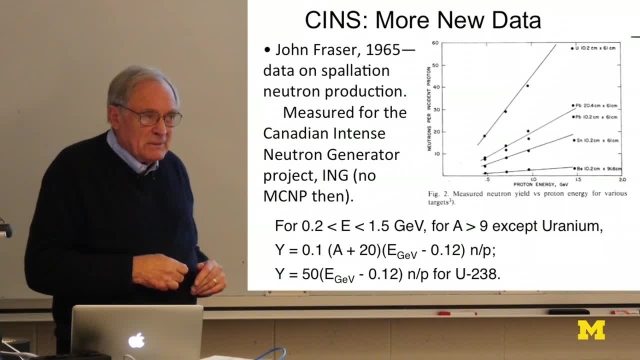 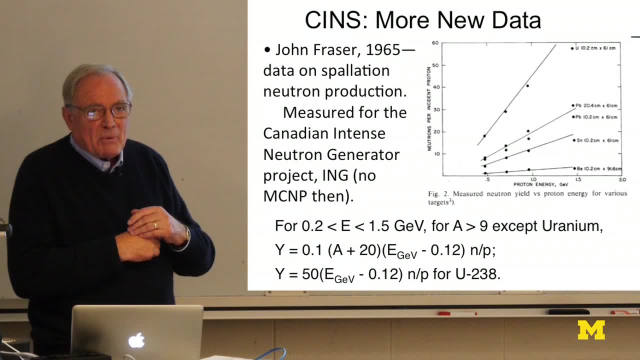 There's another piece of absolutely normalized data And you could put the accelerator performance figures together to know what you could get for proton beams. You could put the target neutron yield figures together to figure what the protons would produce for neutrons, And then you could put Kingsley Graham's neutron yield data together. 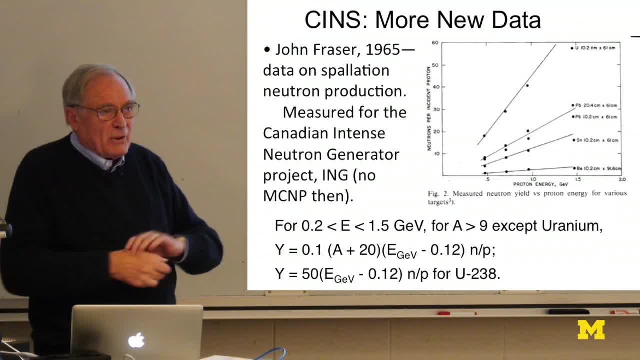 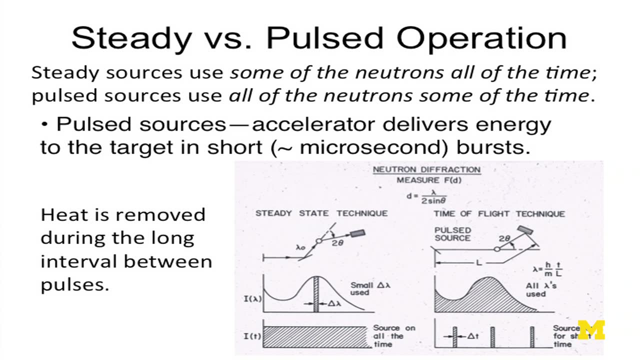 to tell if you had those neutrons or what you could get for a slow neutron beam, And you could design a slow neutron source. So, uh, the committee decided there was a good idea. Furthermore, the sources would be pulsed because the accelerators and synchrotrons 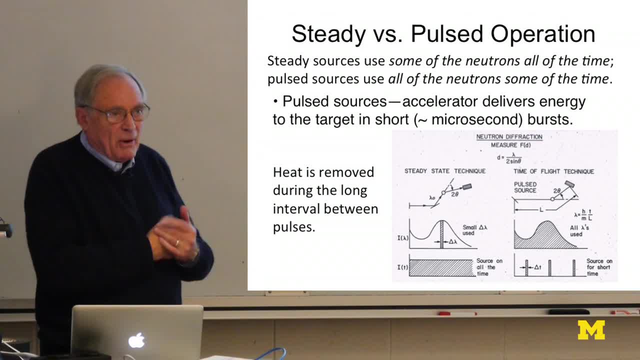 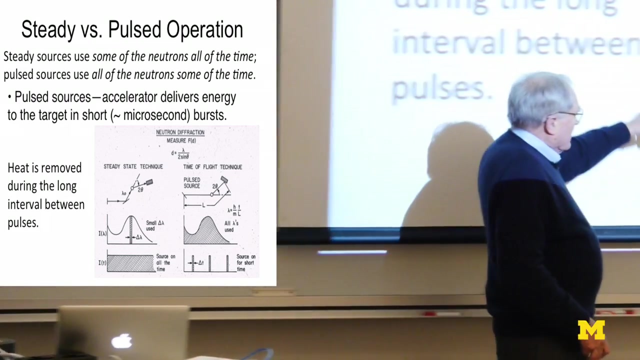 are inherently pulsed machines. So you'd have a pulsed neutron source based on spallation, with time-dependent neutron moderation and hydrogenous moderators. All the work done with reactors, I'll show you. this was usually one from a has a spectrum like this as a function of wavelength. 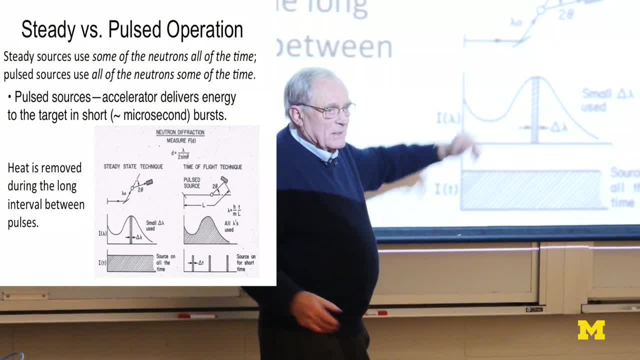 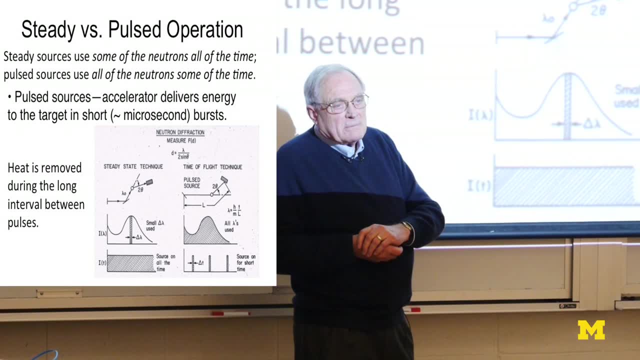 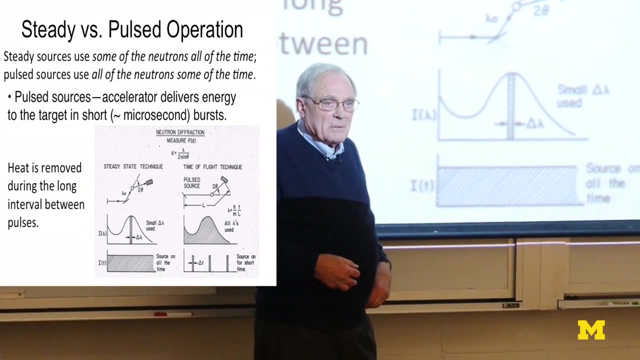 This is the peak for two angstrom neutrons from, say, a water moderator And for work with, say, diffraction, work with a on a reactor beam. you take a very tiny slice out of here and throw the rest away. 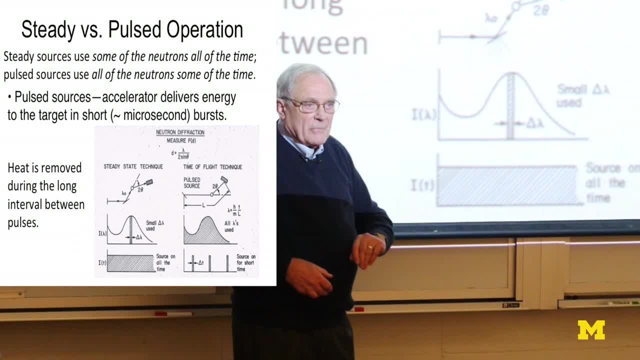 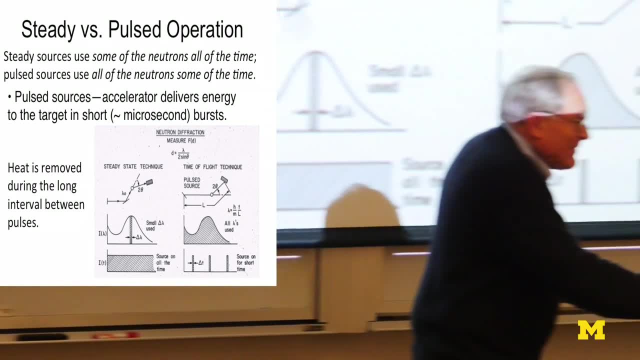 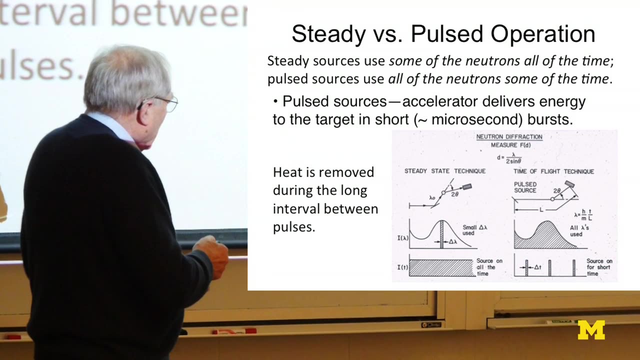 But the reactor is working all the time. This has been a tradition. Oh boy, May I borrow that? Thank you, Yes, So this, Yes, So you take a tiny slice out of the spectrum and you use it all the time. 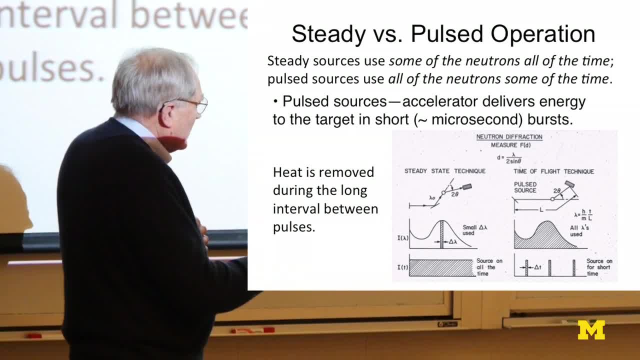 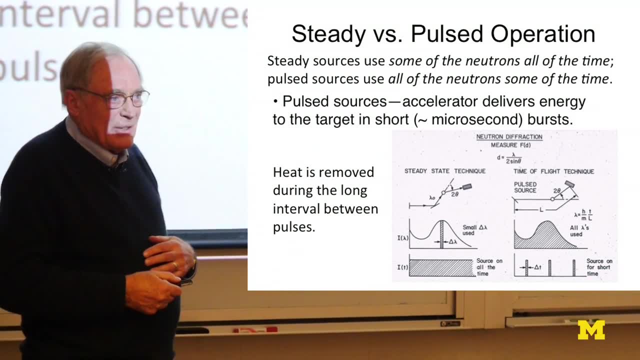 But with the time-of-flight method you measure diffraction by using all the neutrons, but the source is on only a tiny fraction of the time. So you have a duty cycle advantage in that the average comes out to be some small number, but instantaneously. 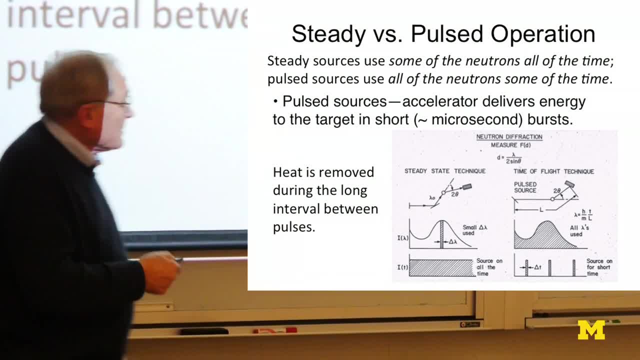 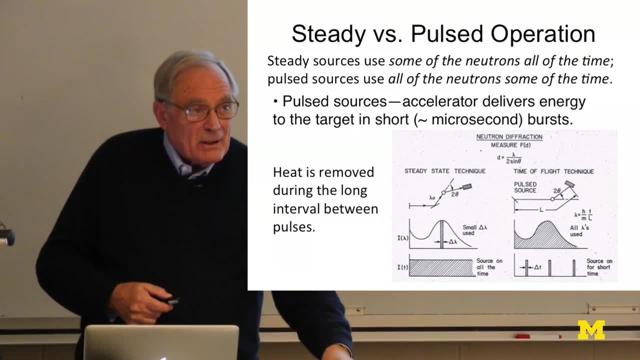 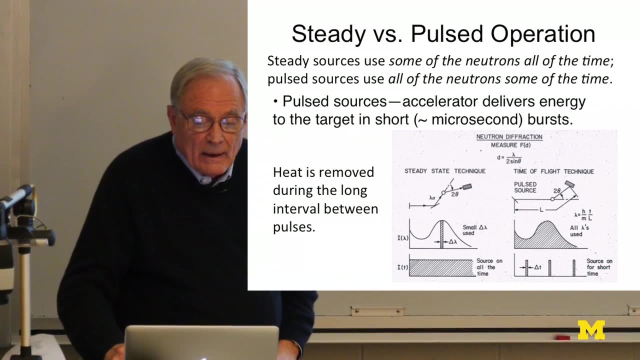 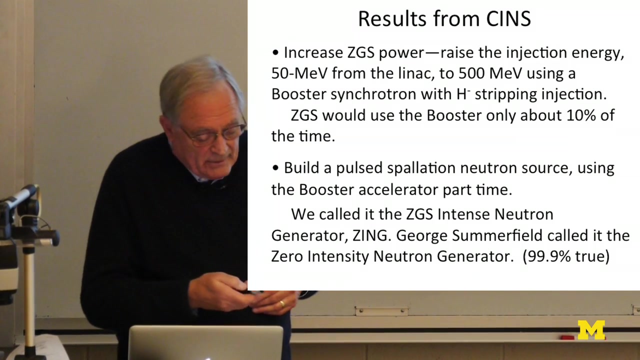 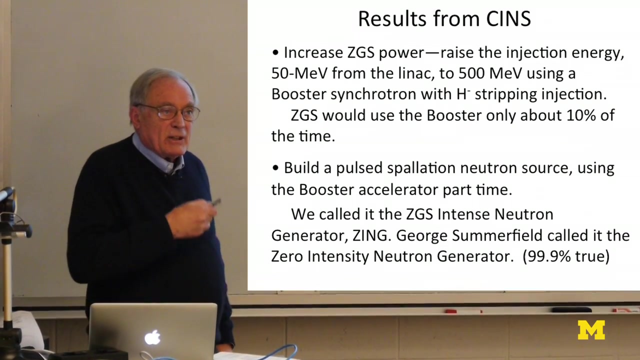 you have a very high intensity. So this makes a pulse source attractive and intrinsically well-suited to an accelerator. So the committee recommended build a new accelerator Instead of injecting it. 50 million volts from a LINAC run the 50 million volt H- ions. into a 500 MeV synchrotron. run this 500 MeV H- ions into the ZGS and strip them there and increase the current in the ZGS. The other recommendation was to build a pulsed-polation neutron source using this booster accelerator. 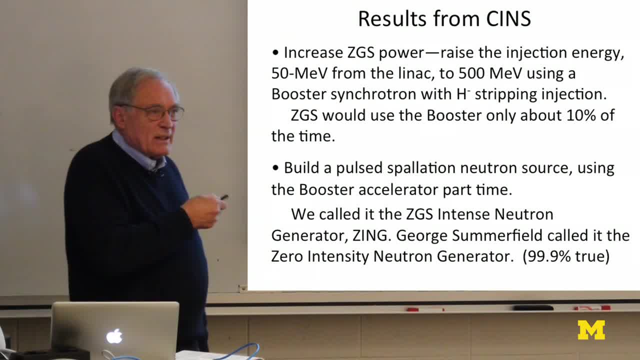 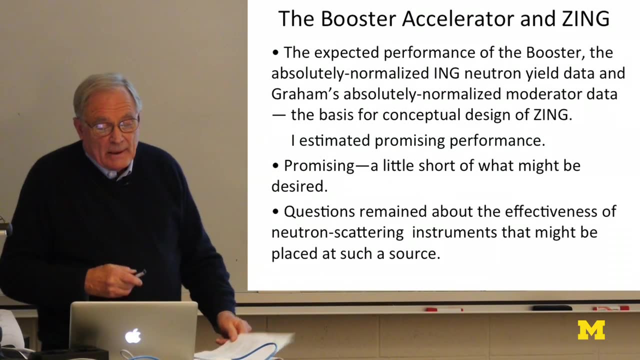 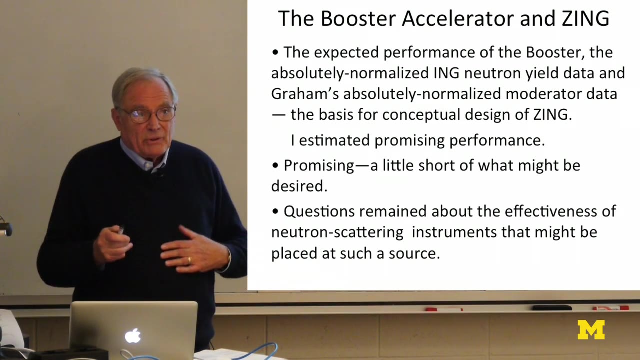 the 500 MeV booster accelerator that was needed for this. Use it part-time to run a slow neutron source, and the recommendation was to do that. So the numbers turned out to be promising, but but they weren't totally convincing. 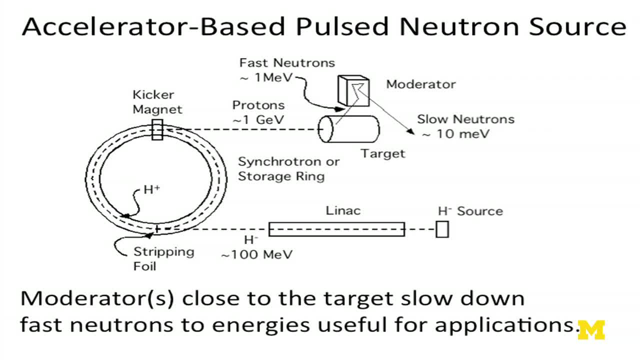 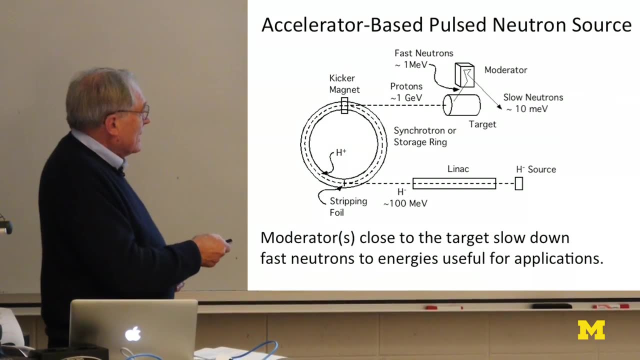 Here's this concept of LINAC: injecting negative hydrogen ions into a ring by stripping protons circulating and increasing in energy in the synchrotron, and coming out at say, say this is in the case that we were doing a 50 MeV or a 100 MeV. 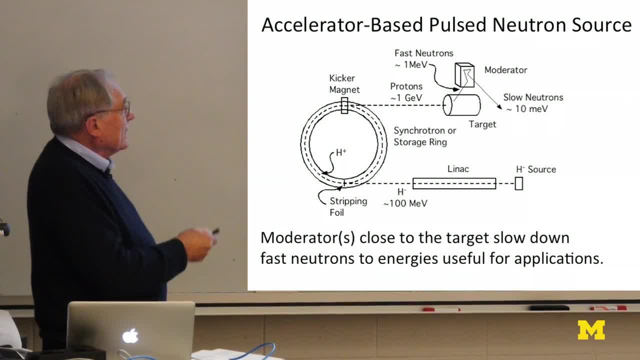 and take them out at 500 MeV or a GeV and let them hit a target. Fast neutrons come out, start moderating in the synchrotron, moderate and produce slow neutron beams with about 10 millielectron volts of energy. 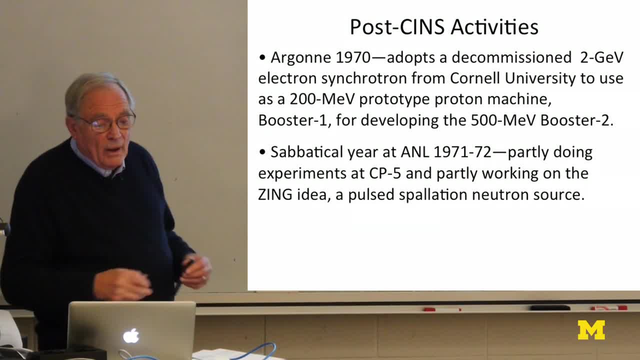 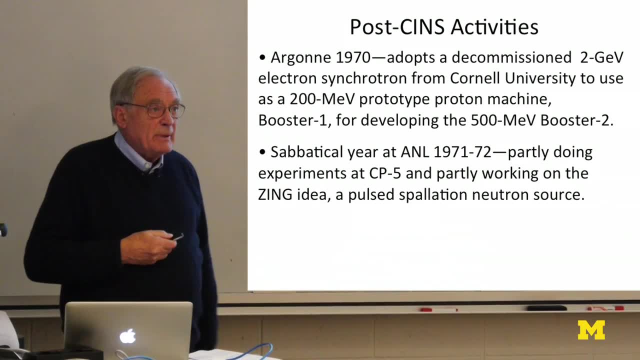 That's the concept And you could. you could do the numbers Today. you would do this with MCNP. There was no MCNP in those days. It was all done on experimental data. So Argonne in 1970, then borrowed. 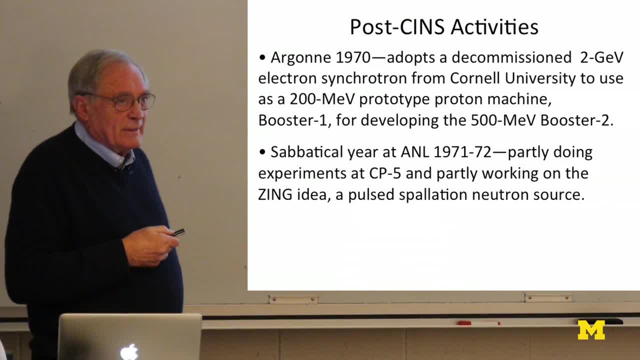 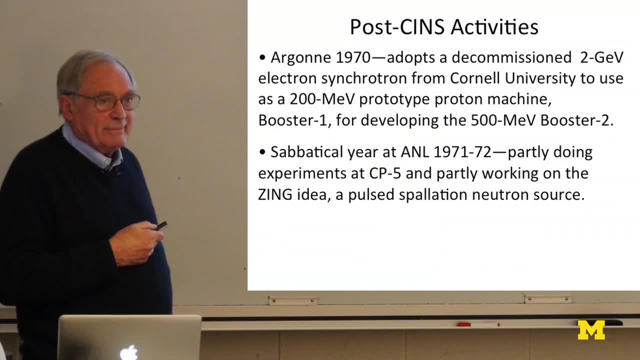 a decommissioned 2 GeV electron machine And they were going to. they converted that into a 200 MeV proton machine for testing purposes And that was called Booster 1.. And in the sabbatical year I spent at Argonne in 1971 and 2. 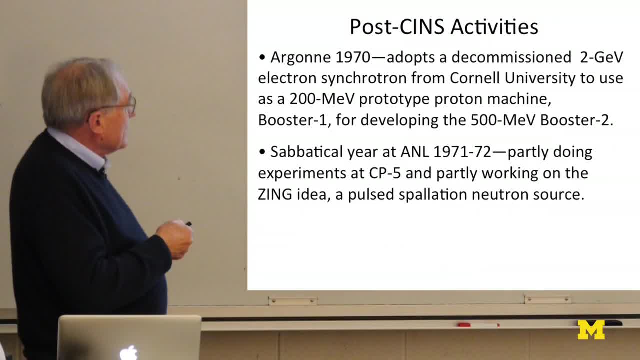 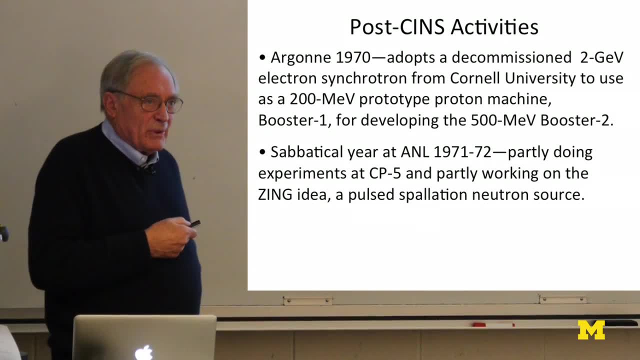 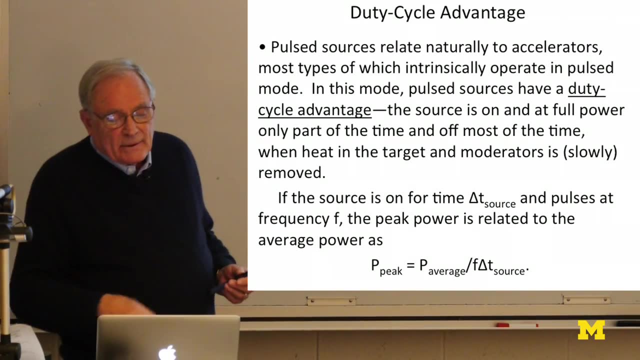 I was doing experiments at the CP5 reactor but working on this idea that we called ZING ZGS Intense Neutron Generator, a Pulse Spallation Neutron Source. So the committee recommended building that. Here's the advantage of running in a pulsed mode. 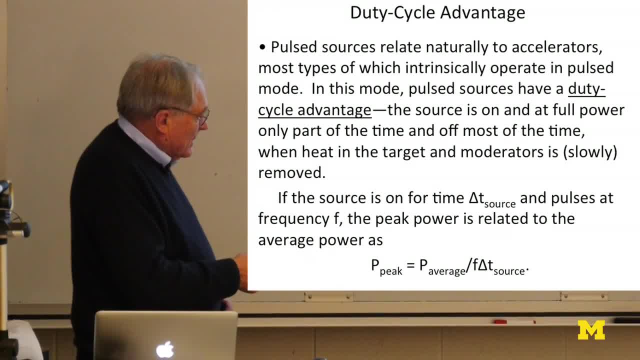 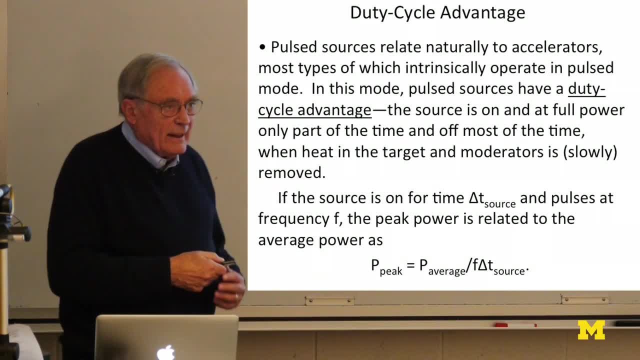 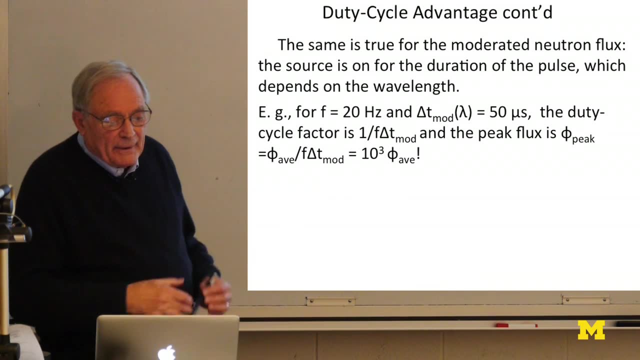 The peak. peak value of the power is the average power divided by the duty cycle factor, which is a product of the frequency times, the source, pulse width, And that number can be like a thousand. And this just does the numbers for a certain case. 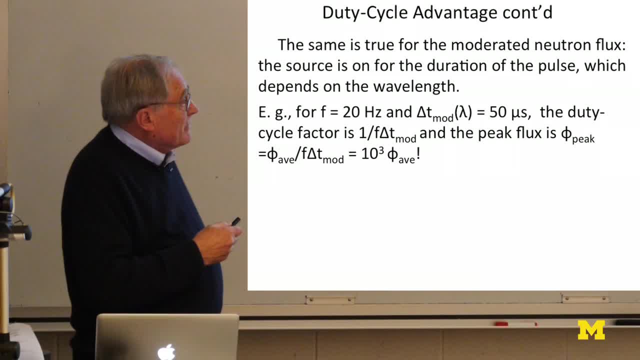 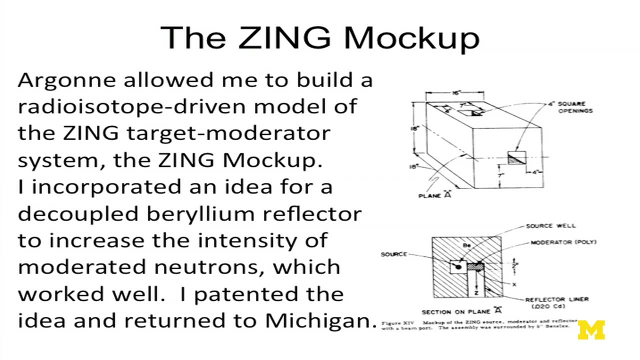 So the duty cycle factor is like a thousand, or it can be ten thousand. The peak value is that much greater than the average value, and the peak value is what counts. So, in order to see what you could do with these ideas while I was at Argonne, 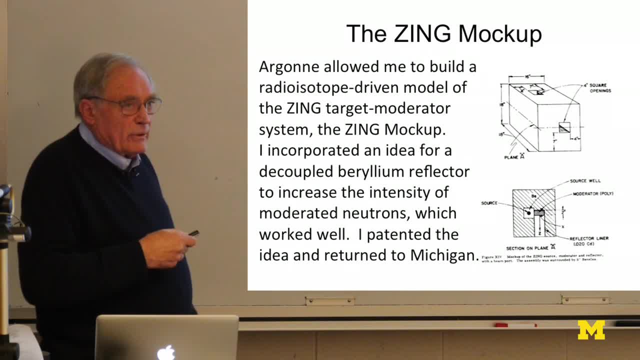 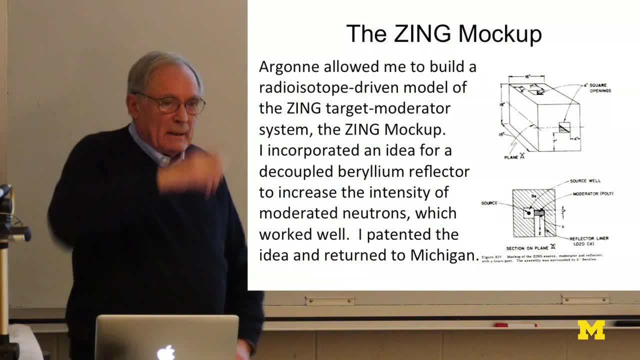 they allowed me to build a mock-up of the innards of the target and moderator system And I could get a pile, a big pile of beryllium blocks which they allowed me to build up Inside. I made a cavity for the neutron source. 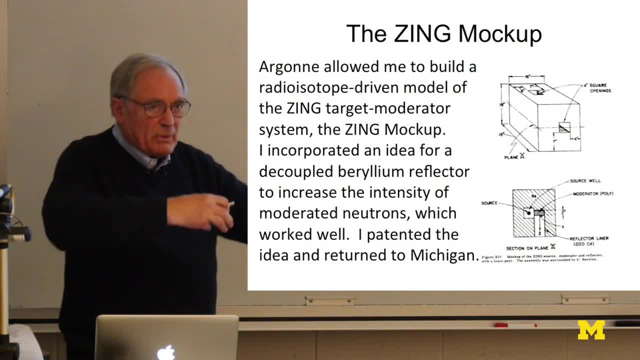 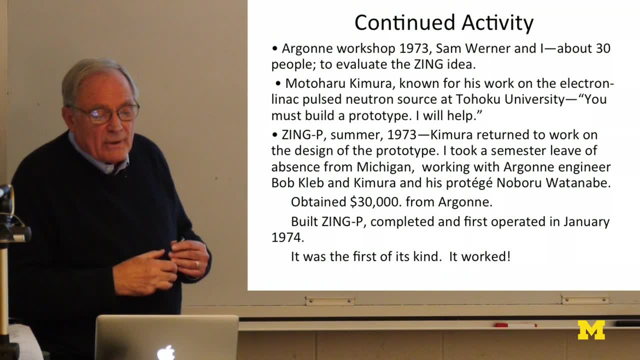 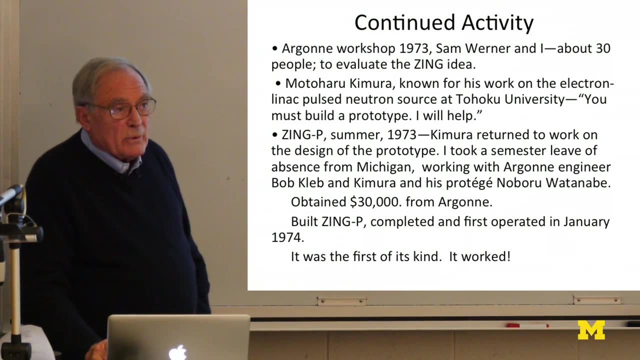 and another cavity for a moderator and cadmium around it to protect it against faster neutrons. So I patented this idea And they gave thirty thousand dollars to to build this. My colleague Kimura, who was at a workshop that that we. 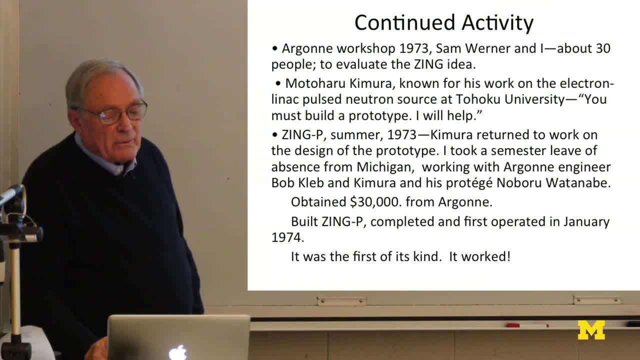 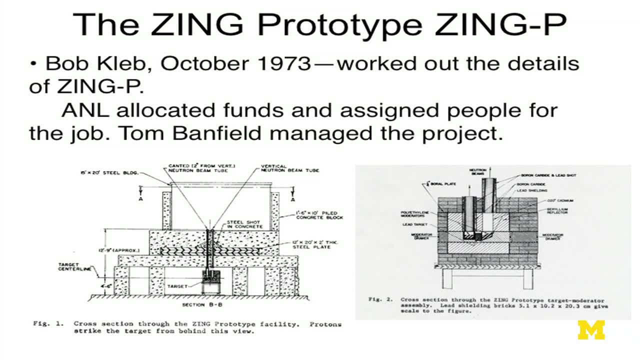 convened to evaluate the ideas. my colleague Motoharu Kimura came to help. Together, we designed a thing that looks like this with a photon beam from a synchrotron. Here was our source. Inside was a lead brick for a target, And 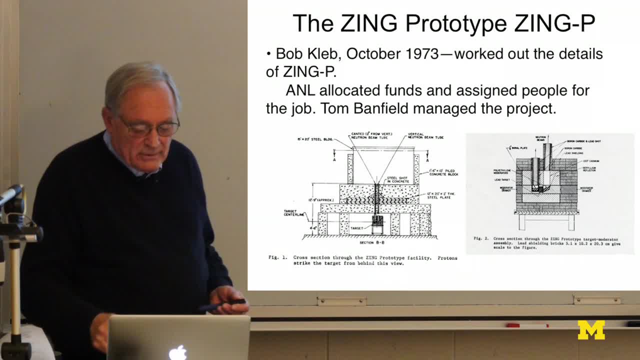 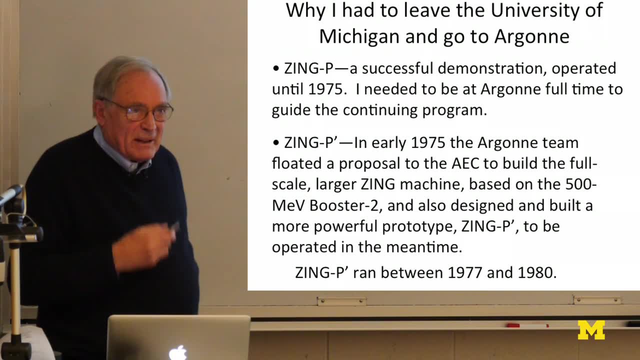 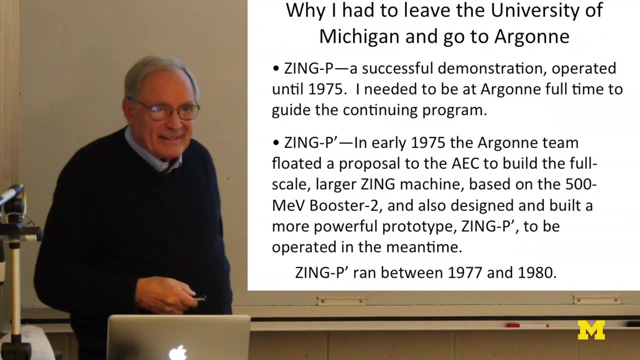 two moderators have produced vertical neutron beams And at that point I've been so involved that I had to leave the university and go to Argonne. So I did that in. I left the university in 1975 to go do that. It was a big risk. 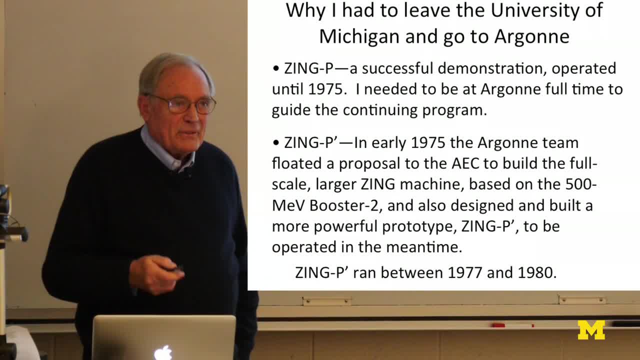 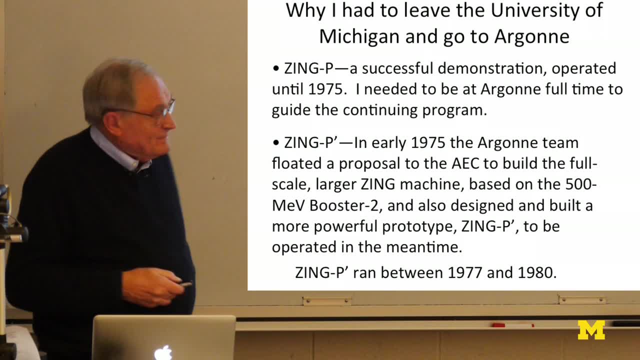 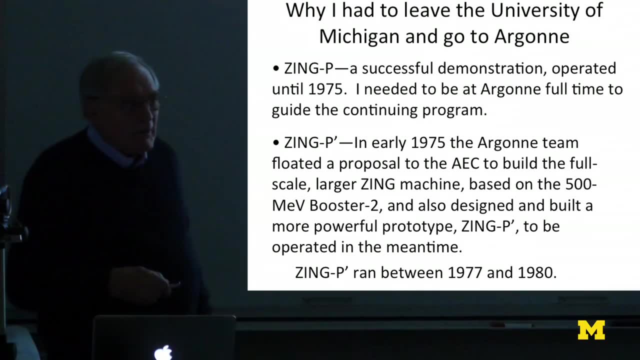 because I loved being here, But I thought that nobody was going to pursue this idea unless I went to Argonne, which I did, And it worked. So we built Zing, And this is the simple one, with the 200 MeV machine. 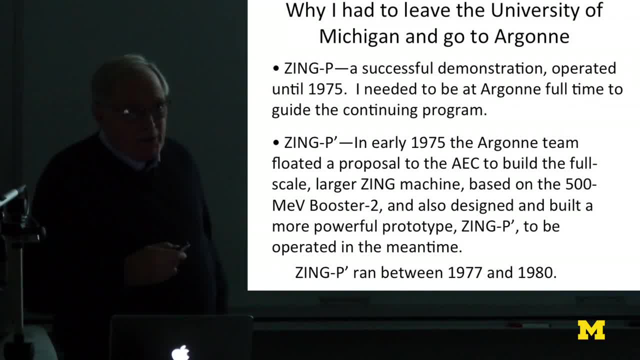 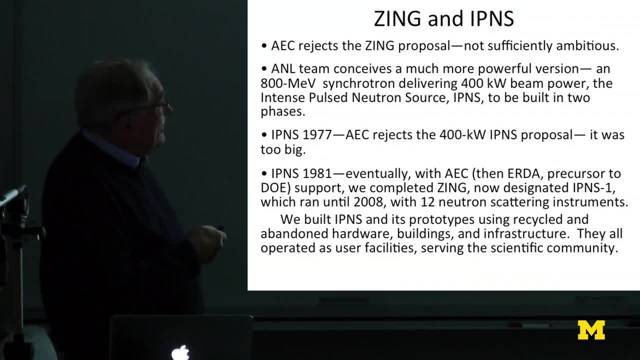 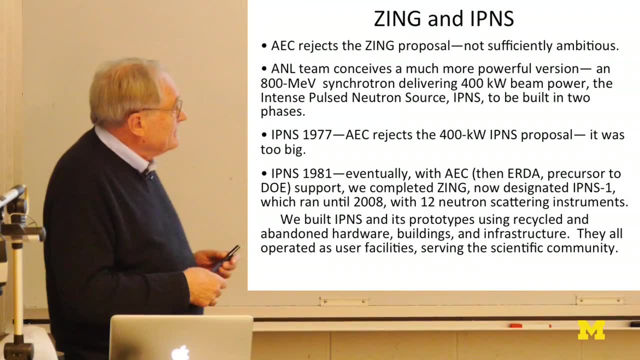 And then we built. when the 500 MeV machine became available, we built, we improved that And that is very productive. Zing P-prime was a very productive research facility And then we worked on what was our big idea, the Zing. 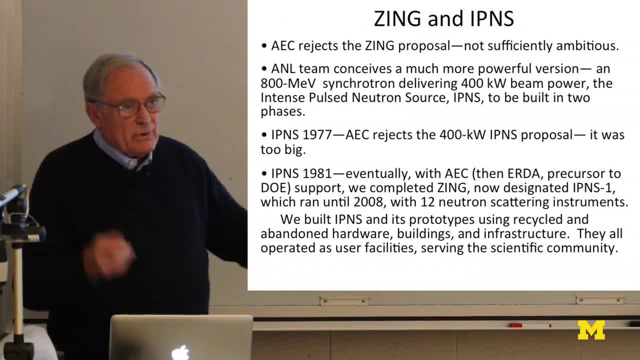 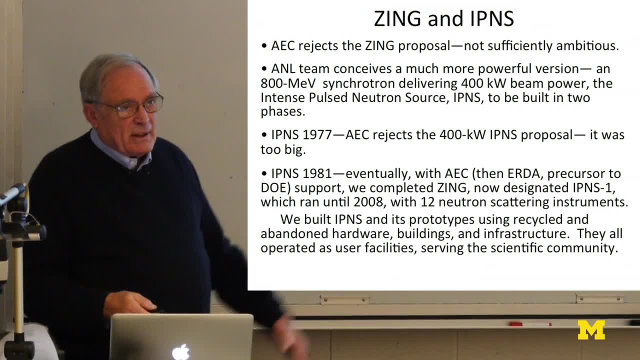 with bigger accelerators and so on. And then we made some proposals to AEC. AEC said: ah, that's not big enough, Give me a better one. So we went and designed a bigger one or a better one And we submitted that. 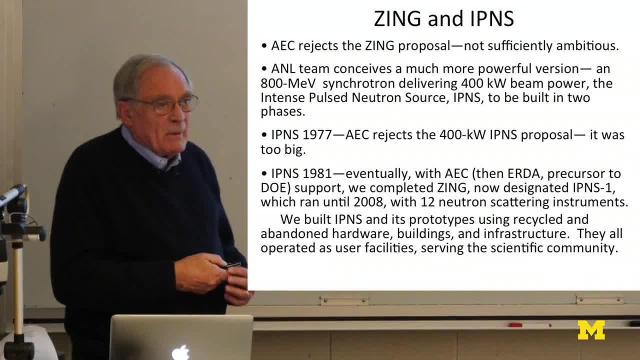 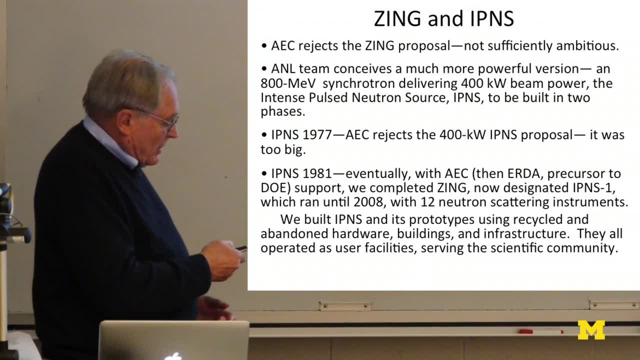 to them and they said: it's too big, Go back again. And we ended up building what was the first thing that we started with And that was called by that time. we called it the Intense Post-Neutron Source- IPNS. 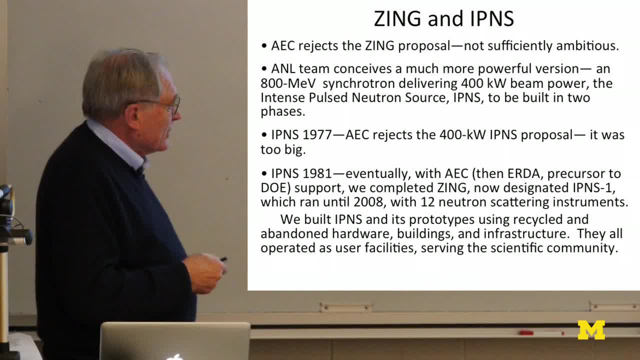 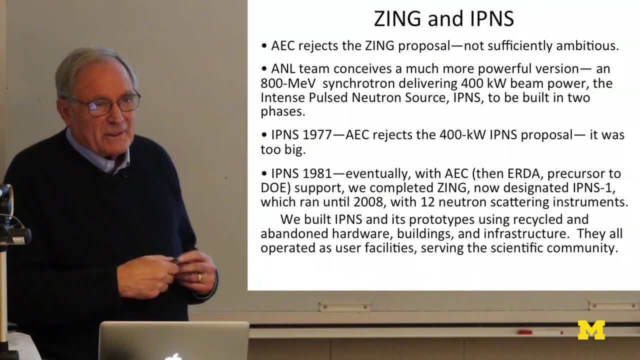 It started running in 1981. And ran until 2008.. And did huge numbers of experiments and did lots of, did lots of science All the time we were using abandoned hardware, recycled buildings and infrastructure that had been built for some other purposes. 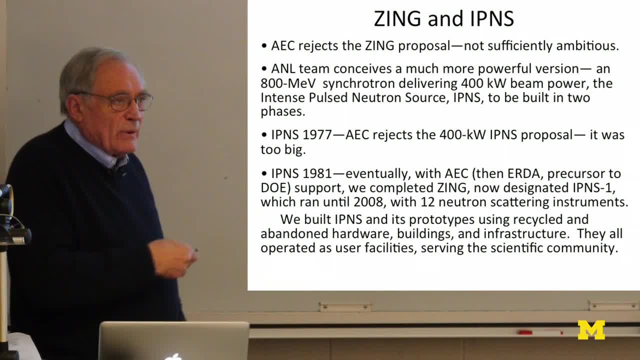 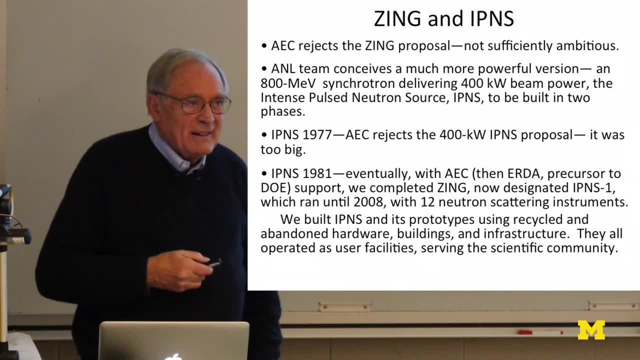 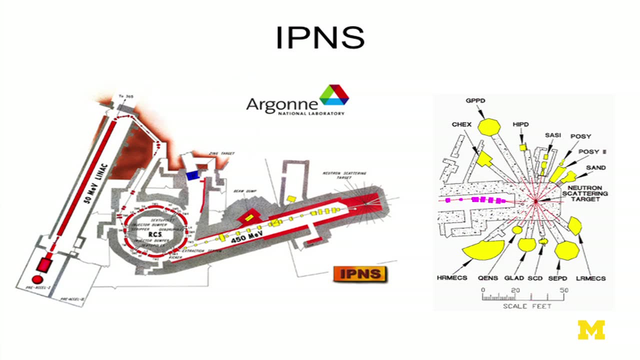 Leftover concrete and iron. So all of this was done on the cheap, using junk, Which is actually a fun way to do things and to have to do them really well. And here's IPNS. This is the 500 MeV machine. 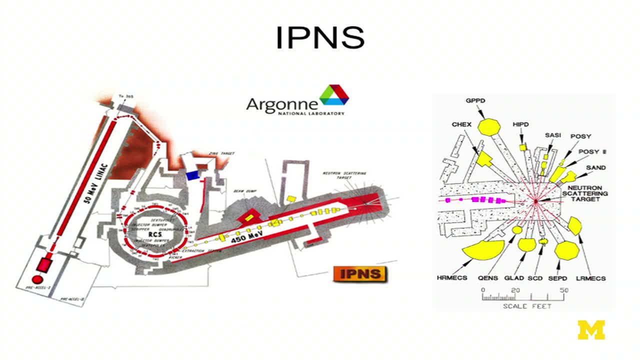 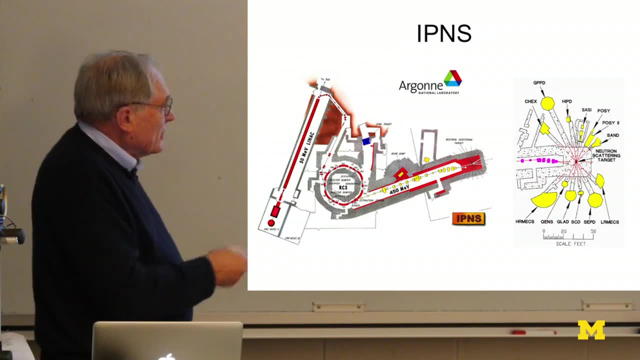 50 MeVh minus LINAC Stripping injection here. Well, we eventually cooled it and ran it 450 MeV. Here's a massive target and neutron source with 12 neutron beams and 12 neutron scattering instruments for neutron science. 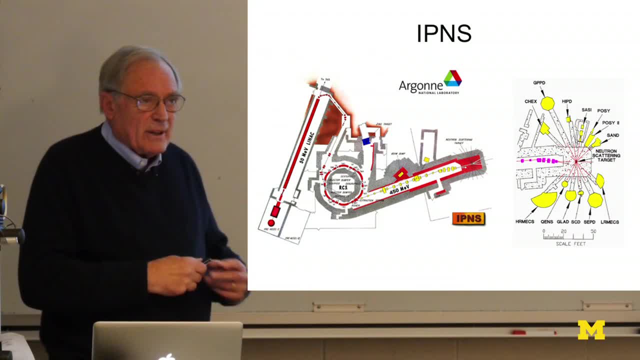 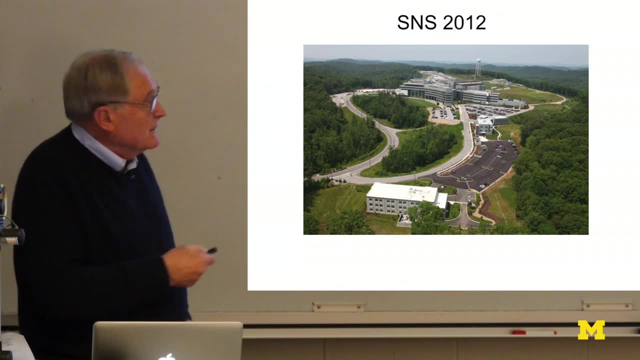 We've gone farther than that now. That was shut down in 2008 because the SNS was completed in 2006 at Oak Ridge And this shows the SNS That will is now delivering. that is now delivering a megawatt. 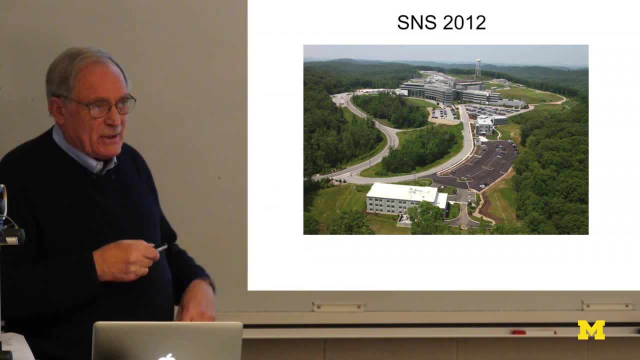 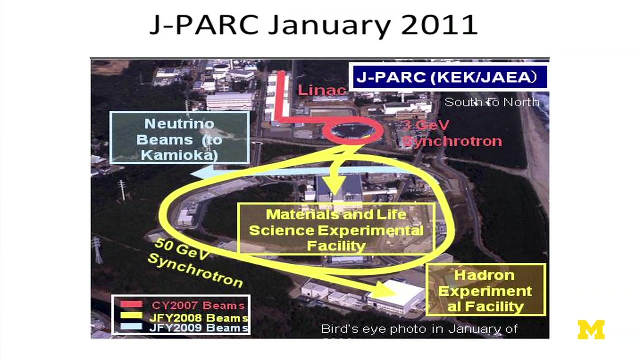 of proton beams in short, pulses less than a microsecond long, 60 times a second. Peak fluxes are like 10 to the 17th neutrons per square centimeter second. Japanese are two years behind and they they've been working with us. 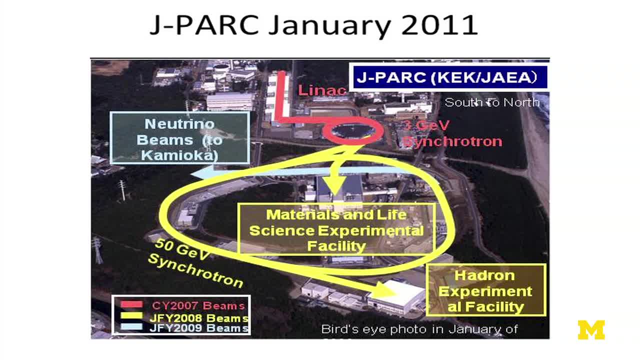 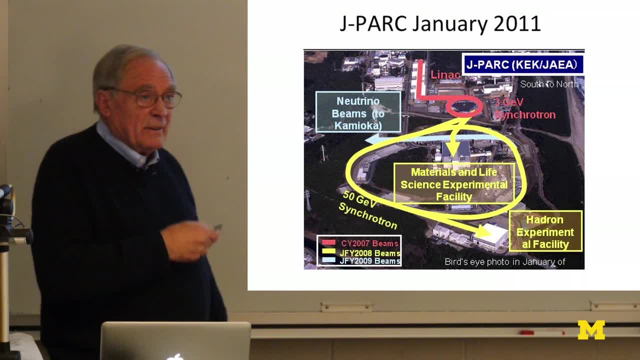 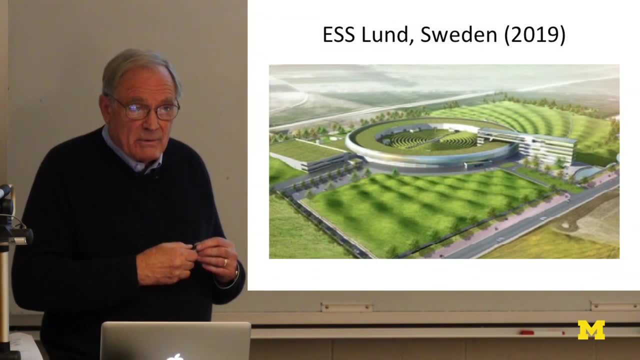 all this time and they built what is called J-PARC, which had several components, and one of them was another one megawatt level spallation source, And under construction now is the European spallation source in Lund, Sweden, which would have five million volt. 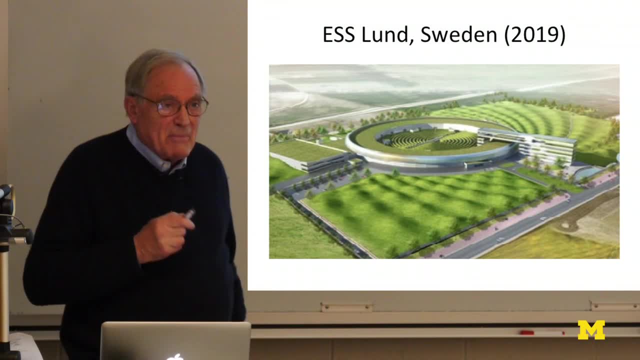 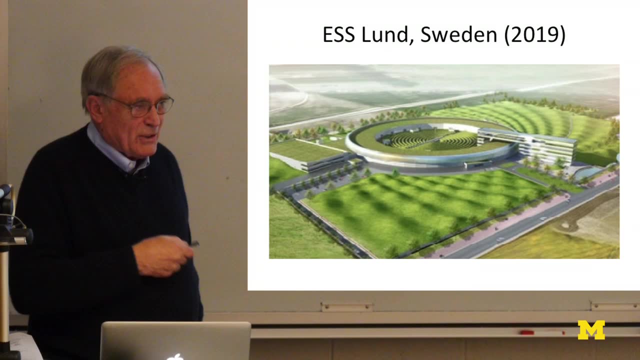 five million watt, five megawatt proton beam cycling at about 15 hertz, using millisecond long pulses. So that's where we have, that's where the technology has gone, And I'll talk a little about other possibilities. You say, if you're going? 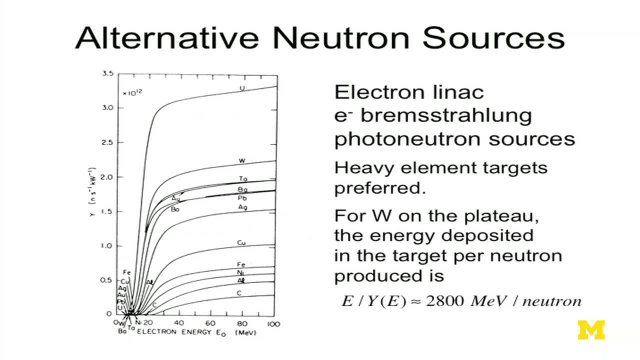 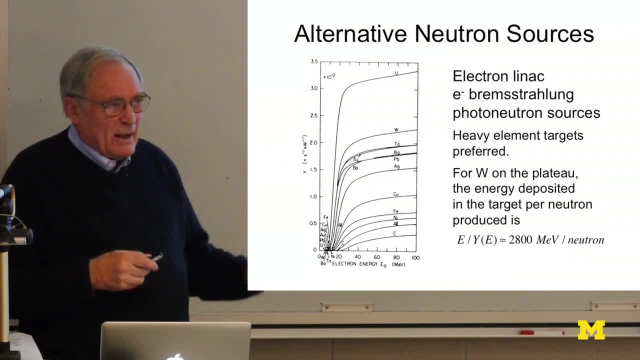 to do all of that. why don't you do it some other way? Everybody's always saying, why don't you do it this way or why don't you do it that way? Well, you really only can do things one way, and there are usually reasons. 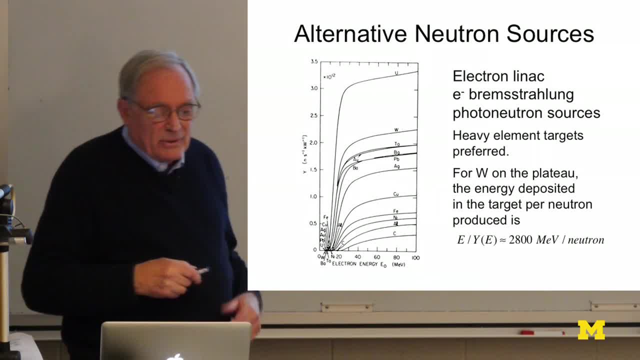 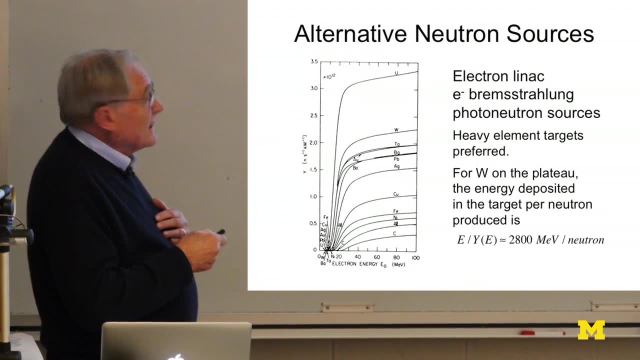 for doing things a certain way, And so you think of the other reasons. One of the one of the popular ways of making pulse neutron sources was electron linear, Say 50 or 100 million volt electrons strike a target, preferably heavy material. Tungsten is nice. 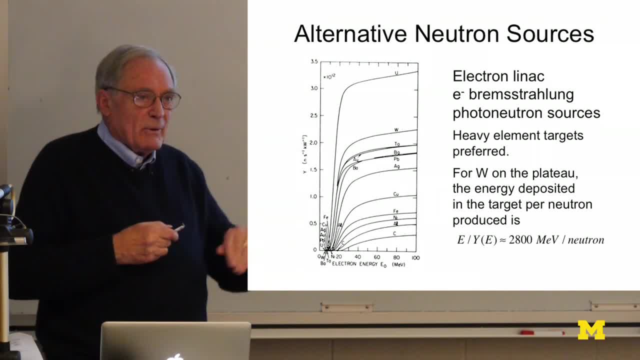 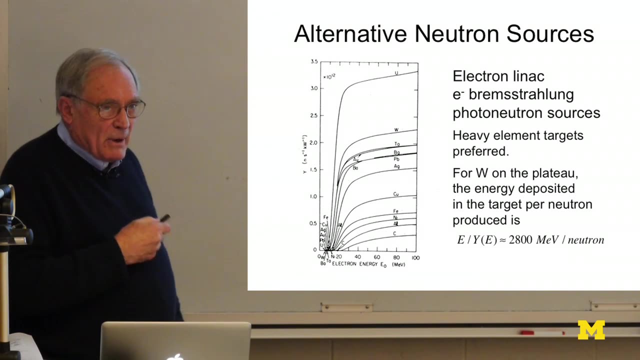 The slowing down the electrons produce gamma rays. Gamma rays interact with the tungsten nuclei through the giant dipole interaction. They heat up the nuclei Nuclei, evaporate neutrons, And this is the principle of photo neutron production by Bram Strahl. in electron linear. This is simple technology. This has been in use since the 1940s, But the yield is so small. yield of neutrons: you have to dissipate almost 3,000 million volts of heat to make one neutron. 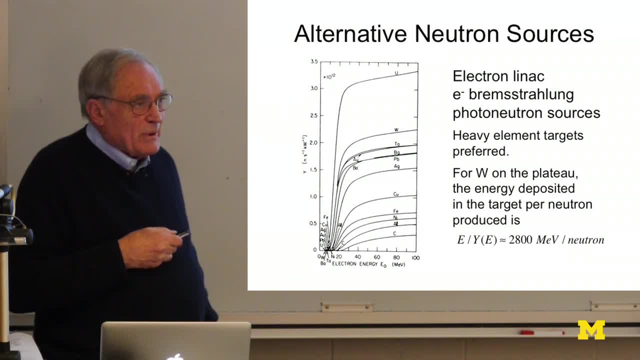 With spallation that number is 30.. 30 MeV instead of 3,000 MeV. So spallation is very efficient, and that's one of the advantages of using a spallation source Instead of electron. Bram Strahl. 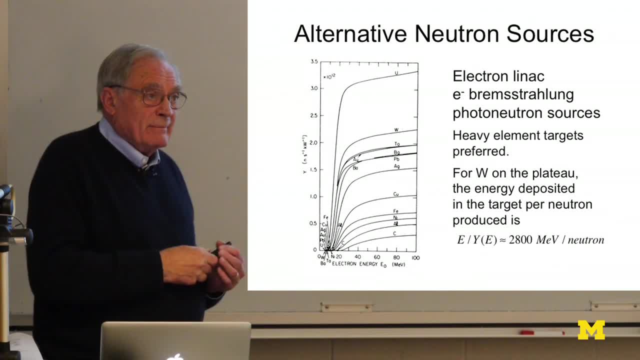 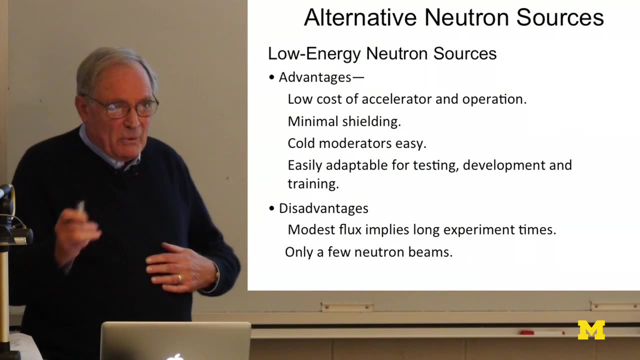 although this is simple, You can do this, But with the power, with a beam of more than 50 kilowatts, you will melt most any target that you have in mind. Otherwise, there are low energy reactions. You are aware here of some of those. 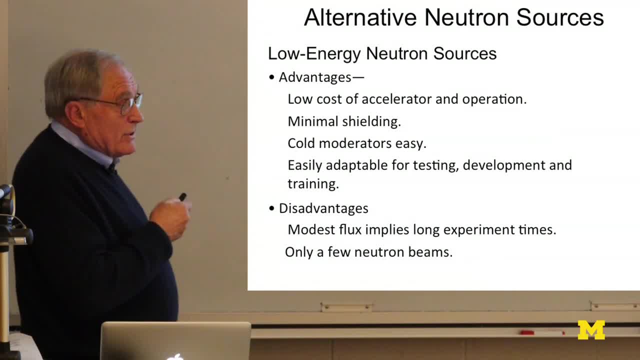 The advantage is that the accelerator- a few million volt accelerator, is effective. this way The accelerator is cheap. Shielding is cheap. Cold moderators are cheap because the fluxes are low. You can easily adapt these because you can't hurt yourself too badly. working around them So you can do testing and development and training and education on using these sources. They are small, Modest fluxes mean if you're doing experiments, the experiments will be long and you will only have a few neutron beams, But these exist. 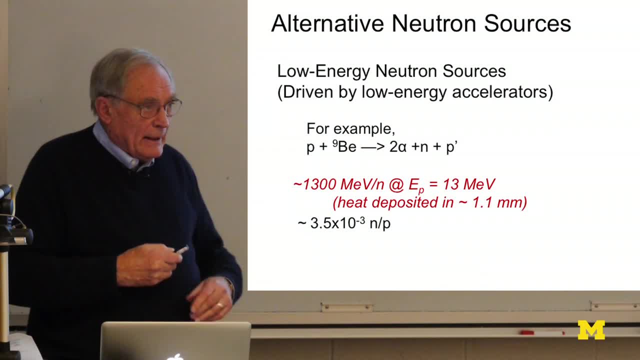 I built one some years ago at MIT. It was a deuterons on beryllium, I think it was, And that was just as a test of building a source for boron neutron capture therapy. But it worked And there's not one operating. 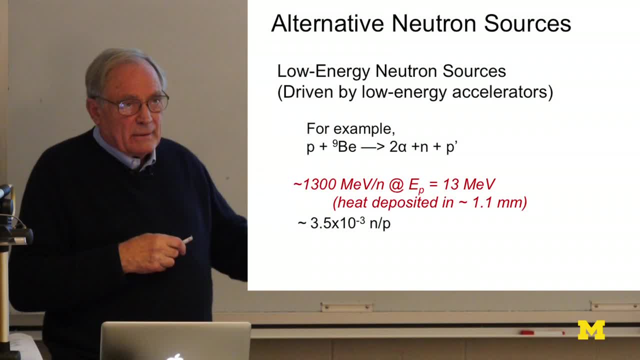 at the University of Indiana by adapting what was the old cyclotron proton cyclotron, Again making something out of junk, And this is called the low energy neutron source. at Indiana, The reaction frequently used is the protons on beryllium. 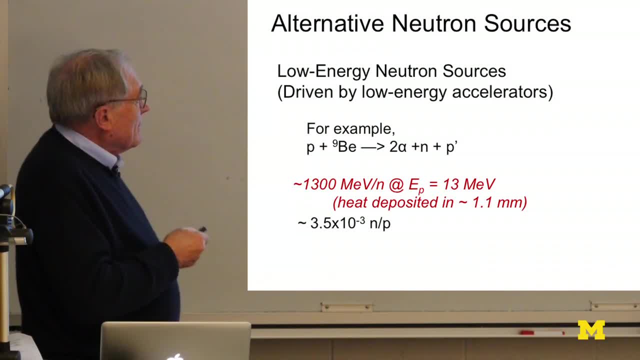 You get neutrons. one neutron per proton. Most of the energy is dissipated, just penetrating the material, But there's a certain amount of neutrons produced And the efficiency, if you wish, is you get about 13,. you have to dissipate. 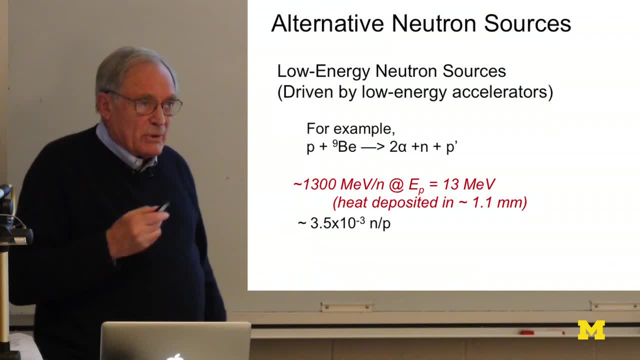 about 1,300 million volts of energy to produce a neutron. But the technology is simple And this means you get three times three or four times 10 to the minus third neutrons per proton. The similar figure for spallation is to get about 30 neutrons. 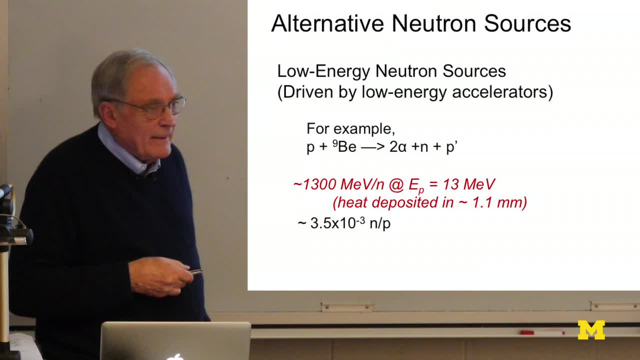 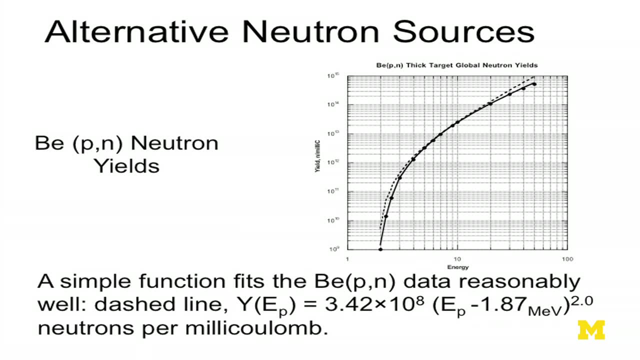 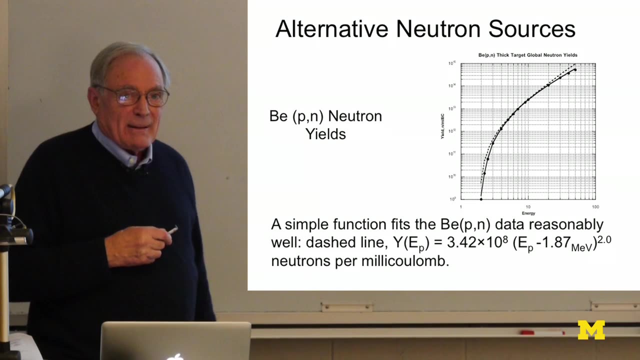 per proton. So nevertheless these are easy and cheap, Good to put in small institutions Bigger than small institutions smaller than you know, major national laboratory Like, for example, university atmosphere. Here's the neutron yield. 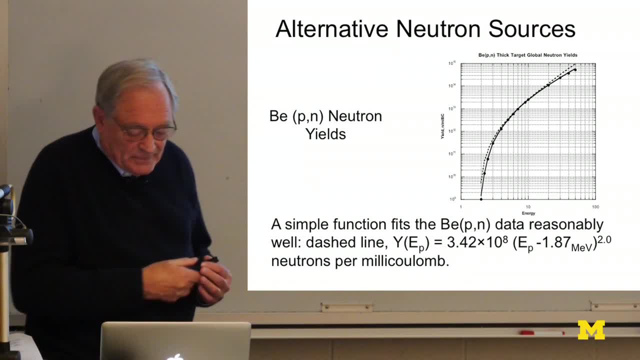 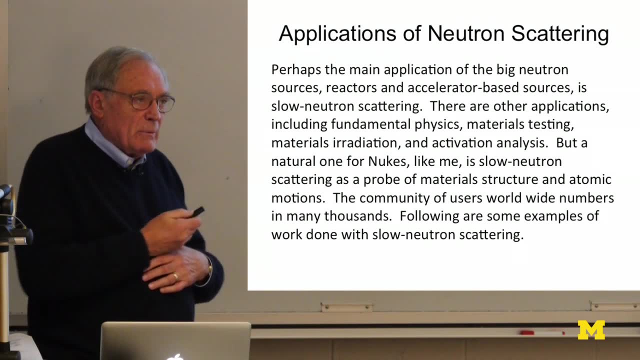 Here's the neutron yield, which I just repeat, for beryllium PN. I think lithium reactions are probably more productive than the beryllium reactions, except that it's hard to deal with lithium. You have to have a window. 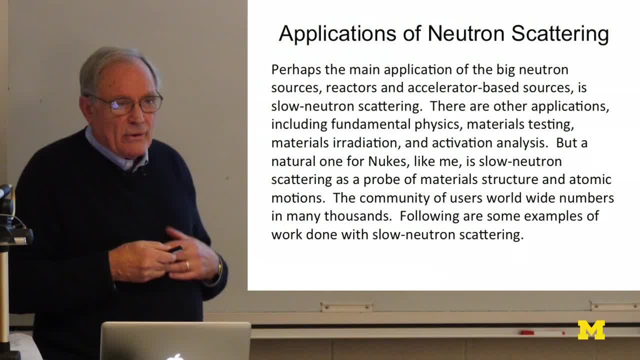 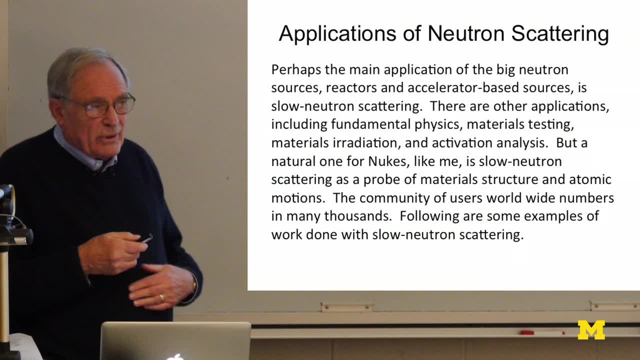 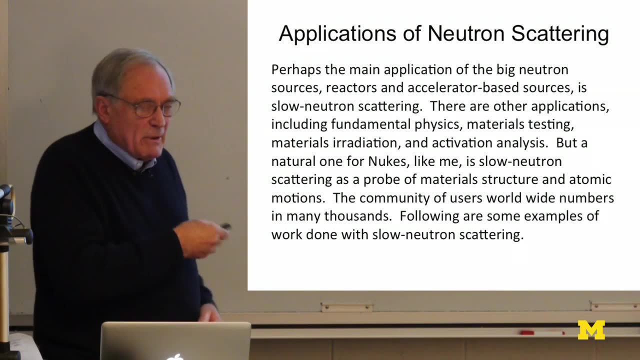 We're talking about low energy particles. They don't go very far through window materials. So really, the lithium reactions. unless you can use a free surface of lithium, which is a hard design problem, this is sort of out. You need to have several MeV. 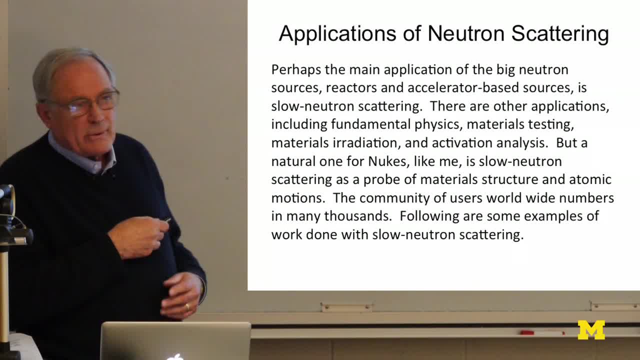 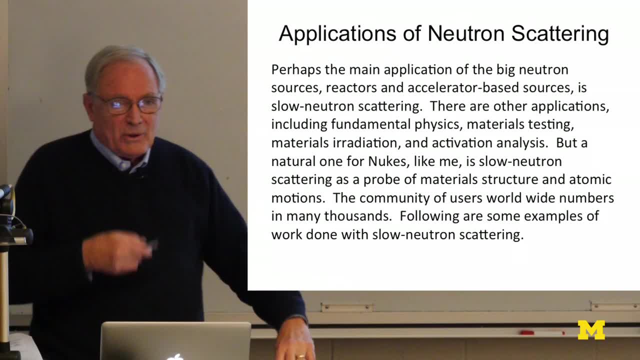 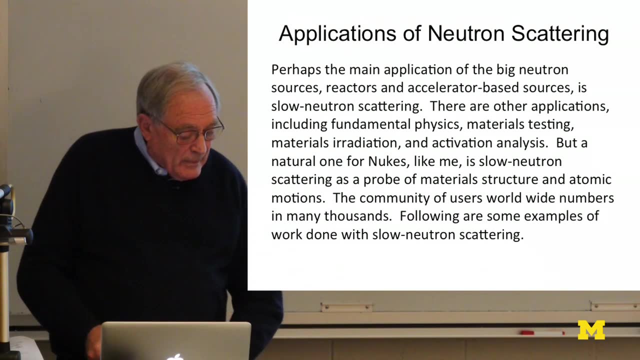 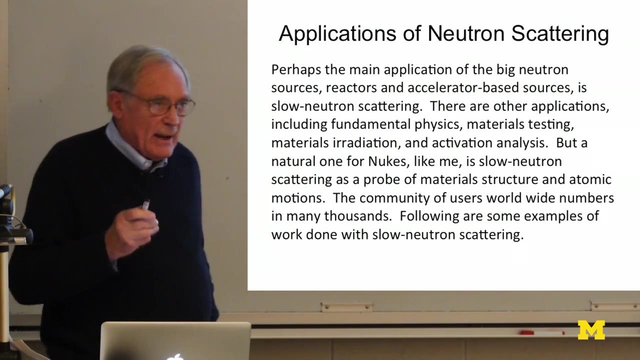 say 10 MeV. protons and beryllium is then the preferred reaction. So what do you do with neutrons if you do have them? I'm turning the subject around a little bit. Here's an example. You do neutron scattering. 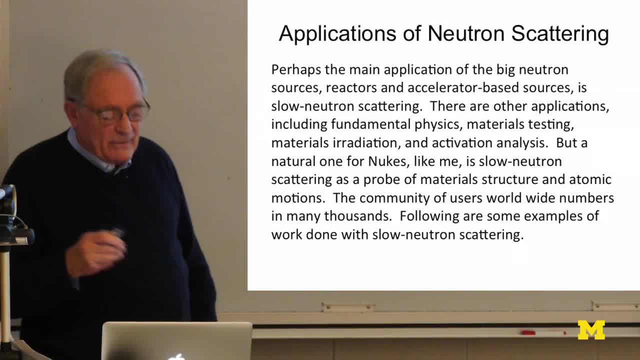 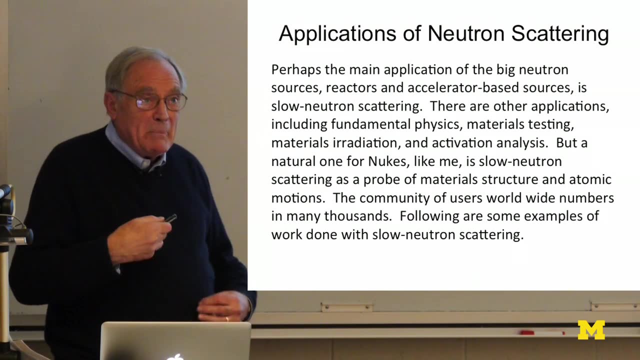 It is the main business of the research neutron sources. For this you need diffractometers or spectrometers of different kinds. I'll illustrate a few, but it's a natural activity for nukes like you and me. There's a lot of the phenomenology. 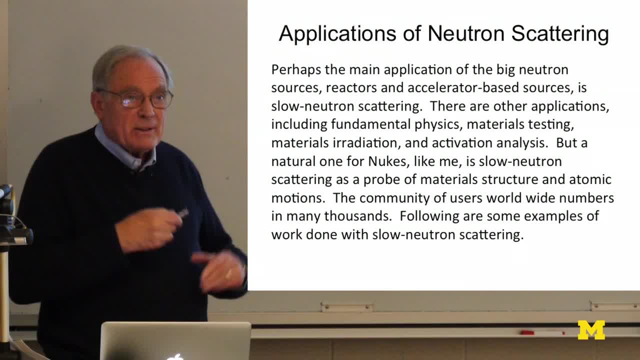 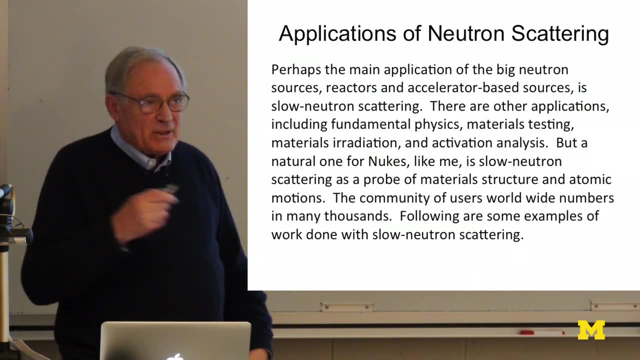 that's important in doing neutron scattering. besides the material science, something material science specialists do is the same grist as we study for other nuclear applications: concept of cross sections and transport of particles and so on. This is natural to all of the nukes. 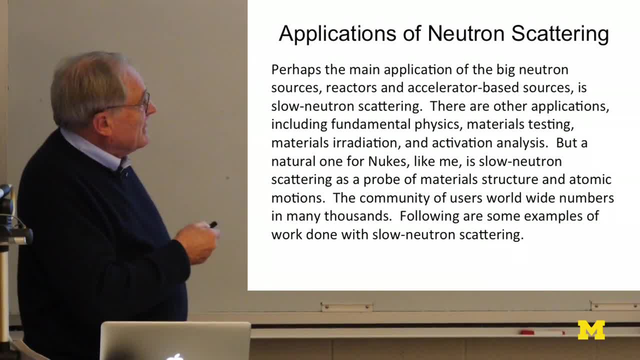 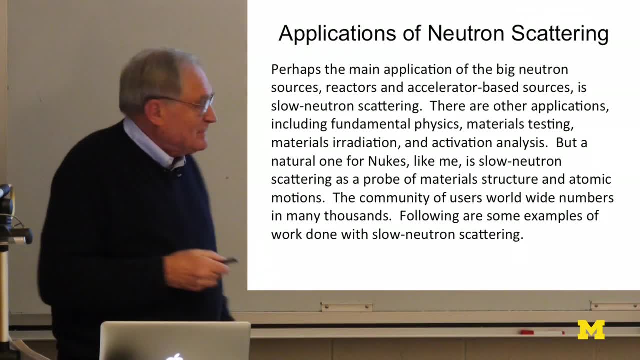 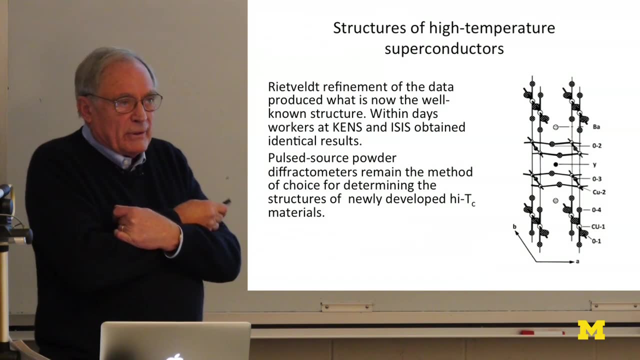 and necessary to do neutron scattering. So this is a nice activity for nukes like you and me. I'll give some examples Early on. when people discovered- 1986,- superconducting properties of ceramic materials, one of the first questions was: 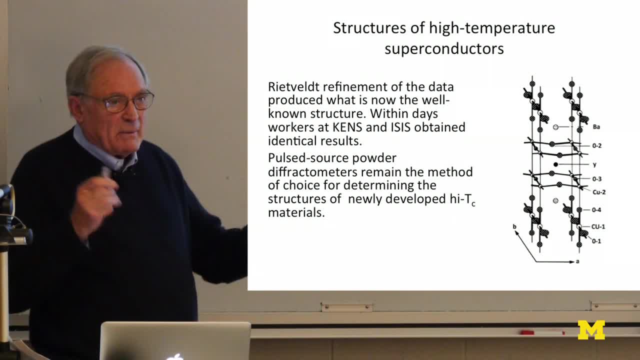 well, why is this Superconducting at about 70 degrees Kelvin was unheard of. It was a huge jump from the highest before, 25 Kelvin, whatever it was. Why is this So? the first question is: what is the structure? 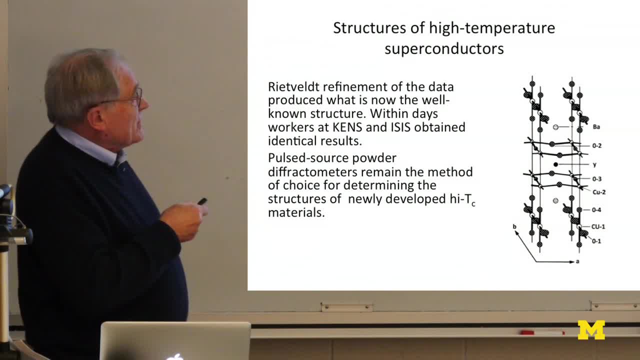 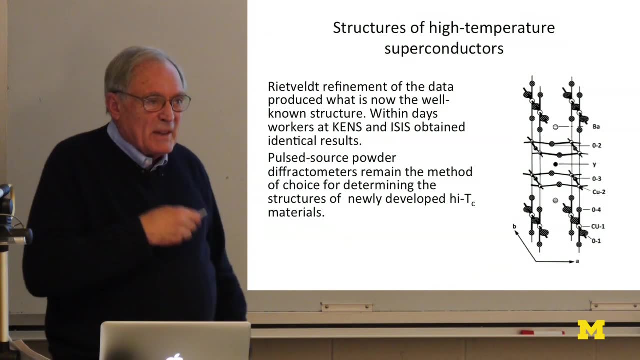 of that material? Well, it consists chemically of copper, oxygen, yttrium and barium, So it's heavy stuff and light stuff. Natural thing for neutrons to do to look for the presence of light atoms in the presence. 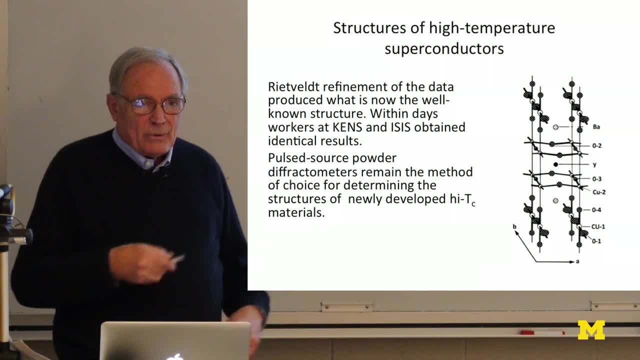 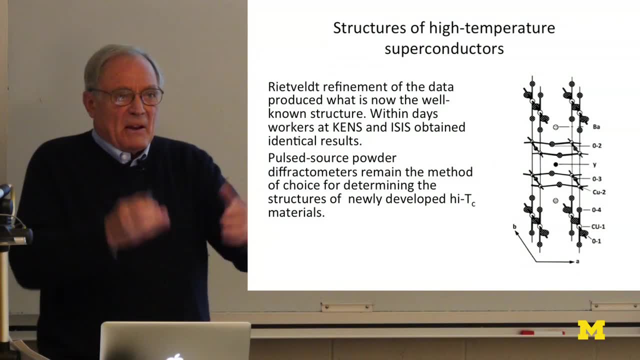 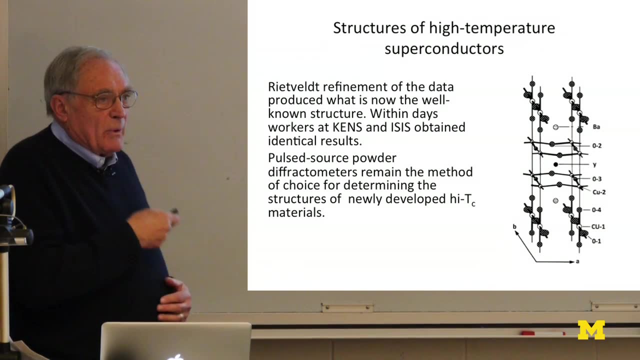 of heavy atoms, because x-rays are overwhelmed by the heavy atoms and neutrons have more or less even-handed scattering properties for all elements, including hydrogen, But in this case it was oxygen, And so our material scientists at Argonne made some samples. 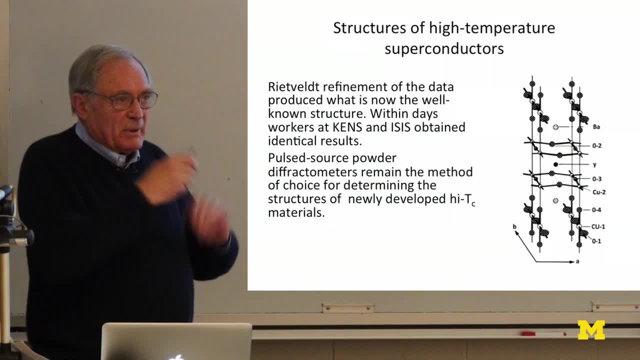 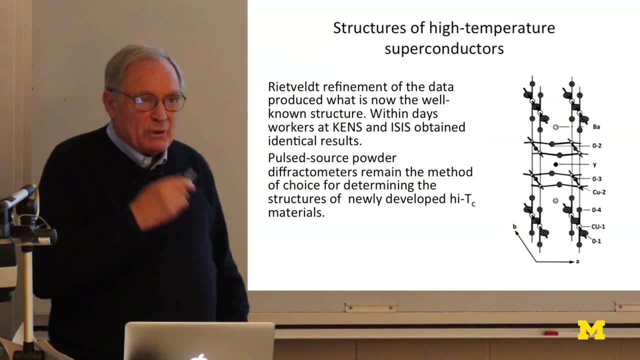 of yttrium, barium, copper oxide. They put in the powder diffracting instrument at IPNS and they determined this structure. It was the first determination of the ITC structure of the material And within a few days the people who had pulse sources. 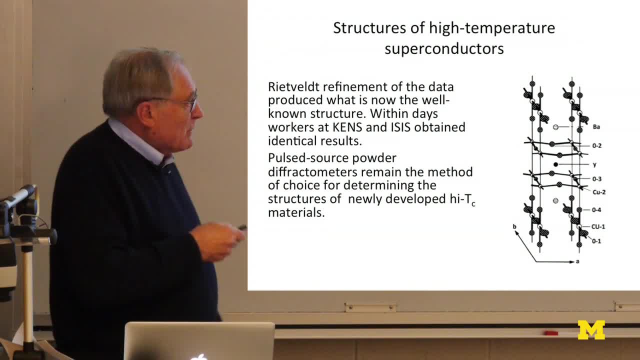 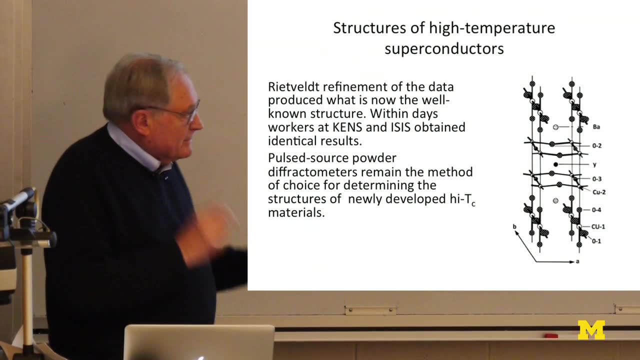 in Japan and in England reproduced the same results, But they're all done on pulse-sourced diffractometers Ever since. when people do new high-temperature superconductors like this, it's the neutron data that they appeal to to know what the structure is. 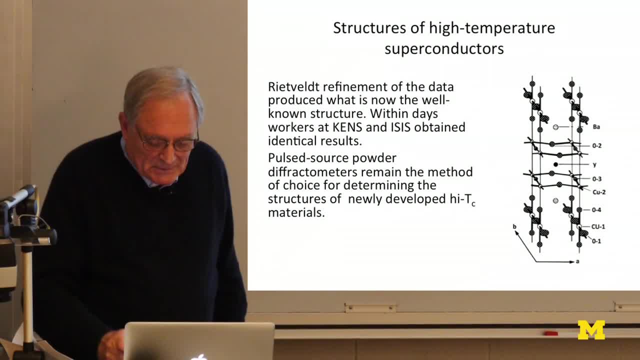 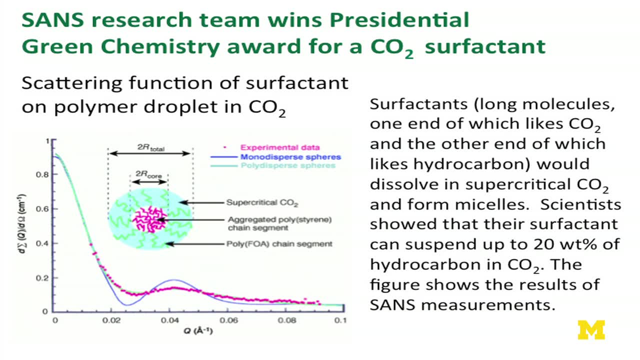 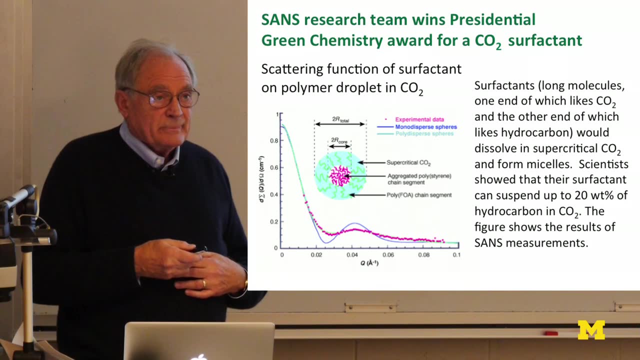 X-rays help, but neutrons are crucial. Here's another one: Green chemistry. There were some people fooling around on the small-angle neutron scattering diffractometer at Oak Ridge using. They were looking for surfactants that were workable in. 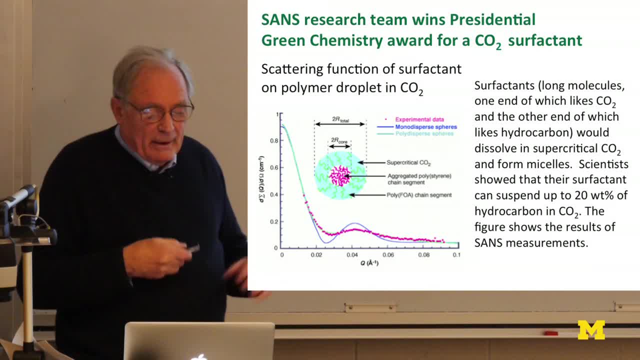 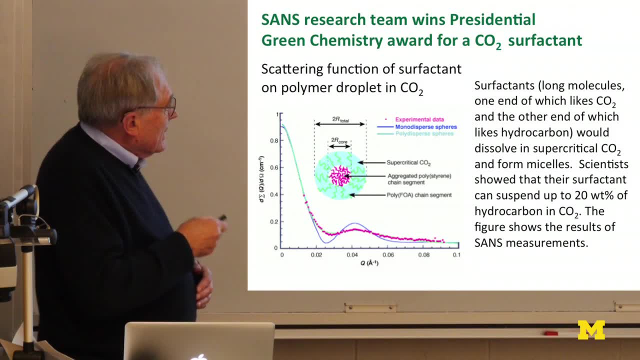 supercritical carbon dioxide And they found some combination that made In a supercritical carbon dioxide- that's room temperature, but high pressure, that's liquid. you could put a polyethylene sphere and this surfactant would surround the spheres and be dispersed inside. 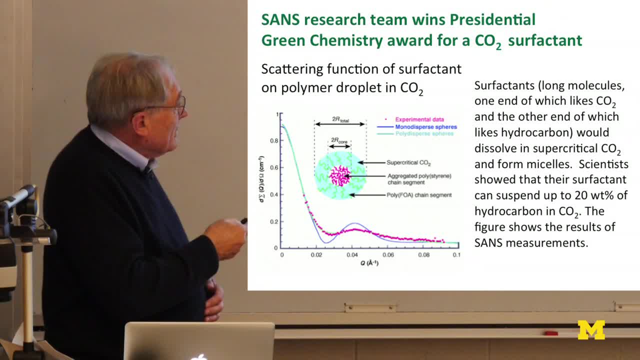 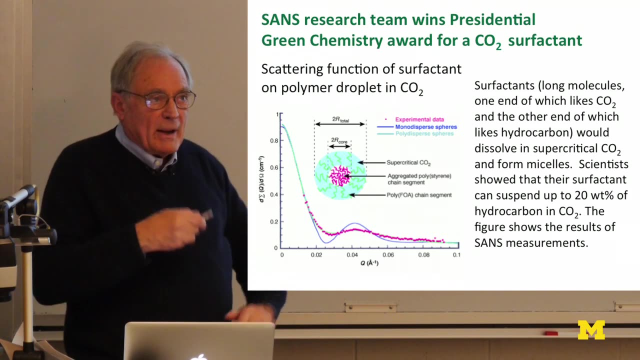 in the carbon dioxide, They formed little micelles like this. This is the principle of dry cleaning or washing machining actually, where surfactants could collect around oil or dirt particles and they'd cause them to float away into the surrounding liquid. So there's a whole industry now. 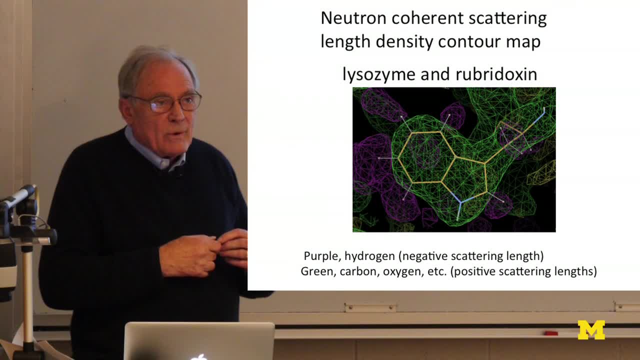 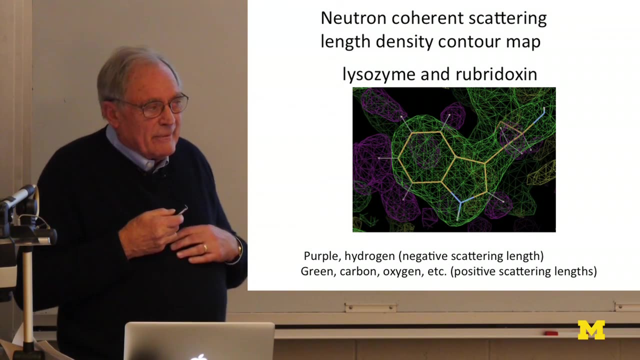 There are hundreds of installations now where they make use of the superconducting- Pardon me, Of the supercritical carbon dioxide surfactants for dry cleaning and displace chlorinated hydrocarbons, which are unpopular when they get into the water system. 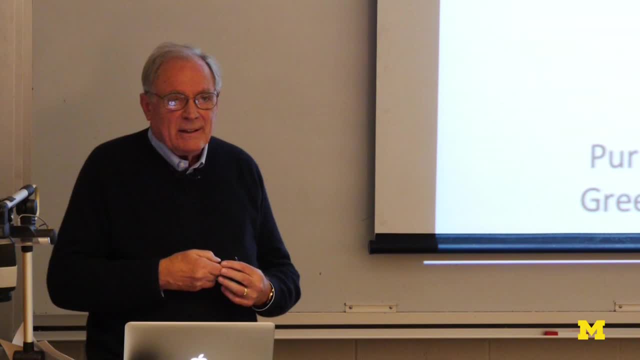 I could go more into it, but neutrons are very useful for material science and that's why we build some of these big machines. I think I'll quit at this point. I give some more examples, but I want to thank you all.